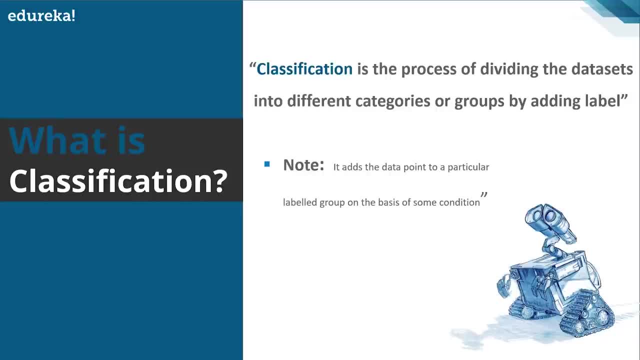 of dividing the data set into different categories or groups by adding label. in other way, You can say that it is a technique of categorizing the observation into different category. So, basically, what you're doing is you're taking the data, analyzing it and, on the basis of some condition. 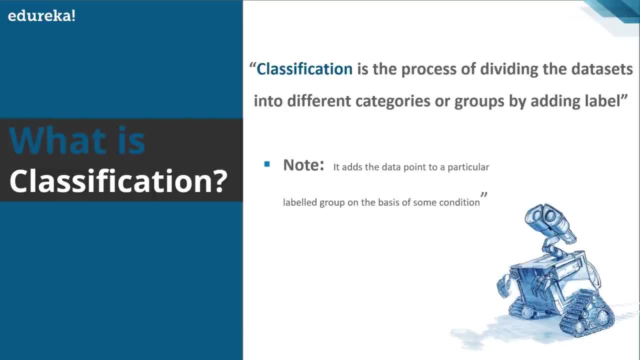 you finally divide into various categories. Now, why do we classify it? Well, we classify it to perform predictive analysis on it, Like when you get the map, you get the data, you get the mail, the machine predicts it to be a spam or not a spam mail And on the basis of that prediction, 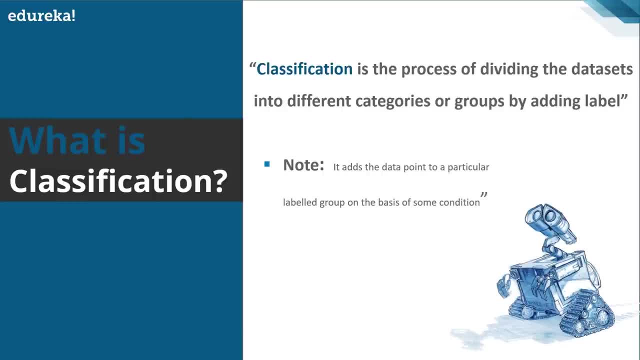 it add the irrelevant or spam mail to the respective folder. In general, this classification algorithm handled questions like: is this data belongs to a category or a B category, Like: is this a male or is this a female, Something like that. Are you getting it? Okay? fine, Now the 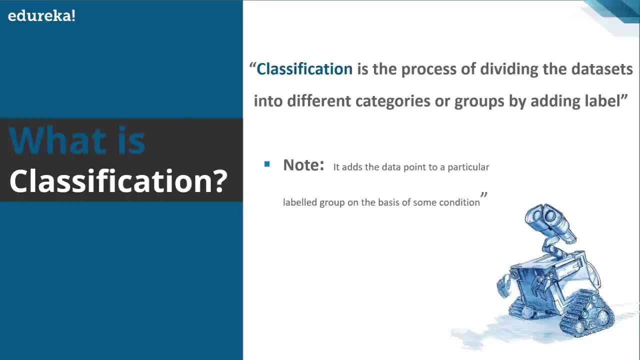 question arises: where will you use it? Well, you can use this for fraud detection or to check whether the transaction is genuine or not. Suppose I'm using a credit card here in India now. due to some reason, I had to fly to Dubai. Now, if, 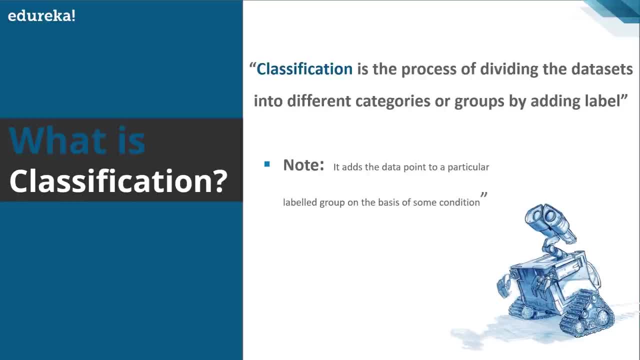 I'm using the credit card over there, I'll get a notification alert regarding my transaction. They would ask me to confirm about the transaction. So there's also kind of predictive analysis, as the machine predicts that something fishy is in the transaction. as very four hour ago I made the 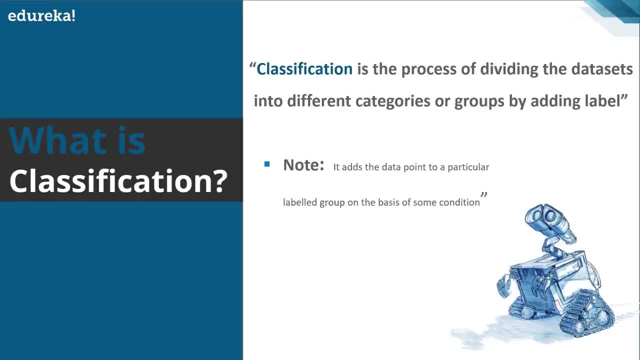 transaction using the same credit card in India and 24 hour later, the same credit card is being used for the payment in Dubai. So the machine predicts that something fishy is going on in the transaction. So, in order to confirm it, it sends you a notification alert. Alright well, this is one of the use case of classification. You 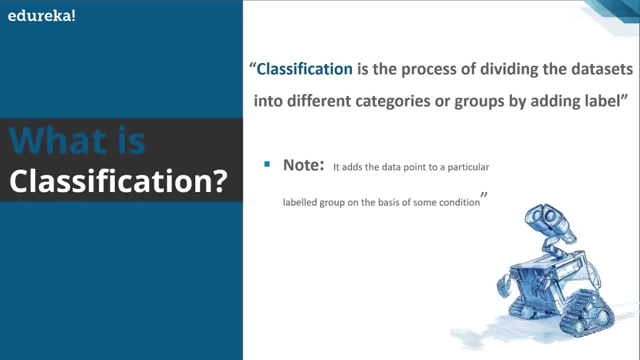 can even use it to classify different items, like fruits, on the basis of its taste, color, size or weight. A machine well trained using the classification algorithm can easily predict the class or the type of fruit whenever new data is given to it. Not just the fruit, it can be any item, It can be a car. 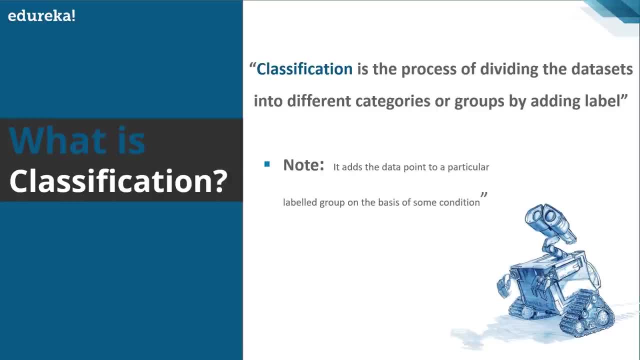 It can be a house, It can be a signboard or anything. Have you noticed that while you visit some sites or you try to log in into some, you get a picture capture for that right Where you have to identify for the given images of a car or it's of a pole or not. You have to select it. For example, there are 10 images and 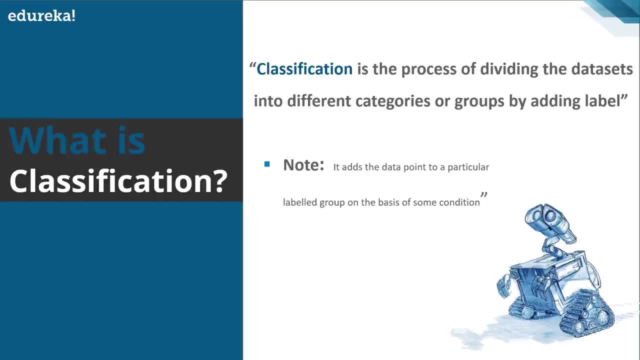 you're selecting three images out of it. So in a way, you are training the machine, right? You're telling that these three are the picture of a car and rest are not. So who knows? you are training it for something big, right. 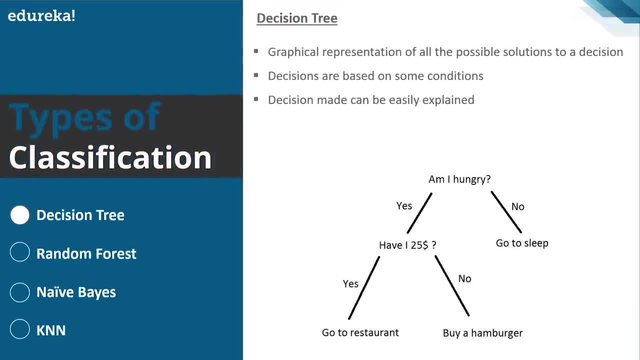 So, moving on ahead, Let's discuss the types of classification, All right? Well, there are several different ways to perform a same task, like, in order to predict with a given person is a male or a female, The machine had to be trained first, All right, but there are multiple ways to train the machine and you can choose any. 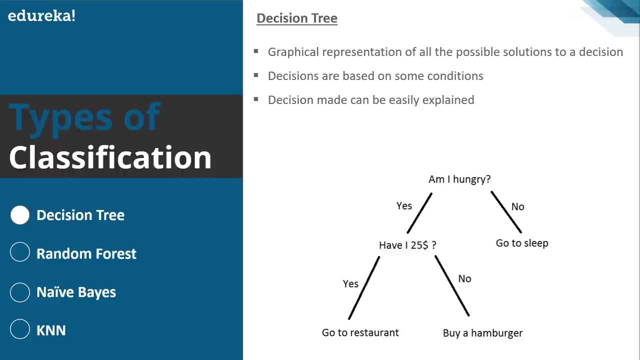 one of them just for predictive analytics. There are many different techniques, but the most common of them all is the decision tree, which will cover in depth in today's session. So as a part of classification algorithm, we have decision tree. random forest name buys. 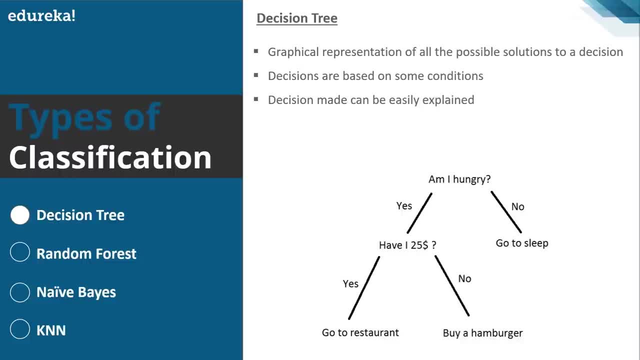 K, nearest neighbor- logistic regression, linear regression, support vector machines, and so on. There are many, All right, so let me give you an idea about few of them, starting with decision tree. Well, decision tree is a graphical representation of all the possible solution to a decision: The decisions. 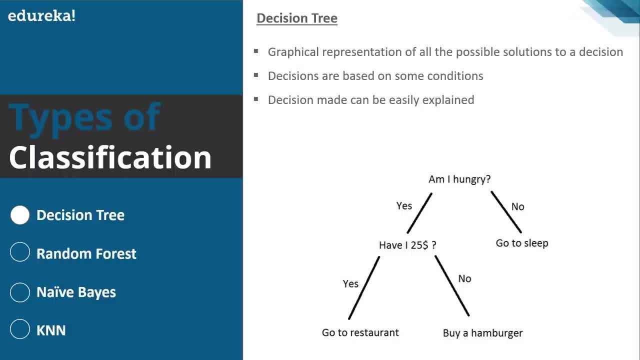 which are made. they can be explained very easily. For example, here is a task which says that: should I go to a restaurant or should I buy a hamburger? You are confused on that, So for that, what you will do will create a decision tree. 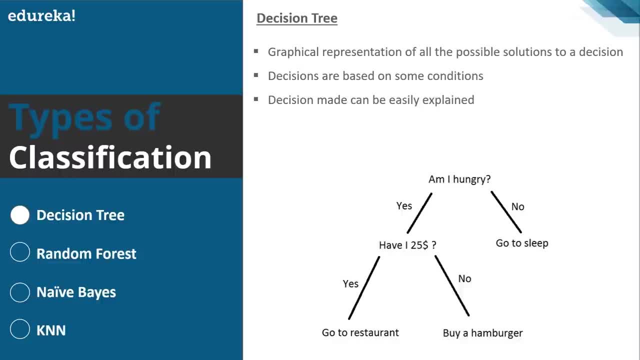 For it. starting with the root node will be: first of all, you'll check whether you are hungry or not. All right, if you're not hungry, then just go back to sleep, right? If you are hungry and you have $25, then you will decide to go to restaurant. And if you're hungry and you don't have, 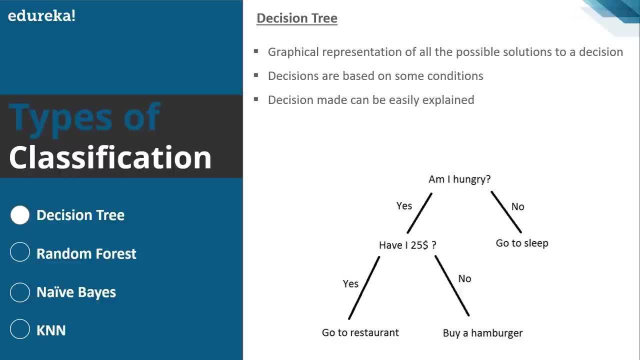 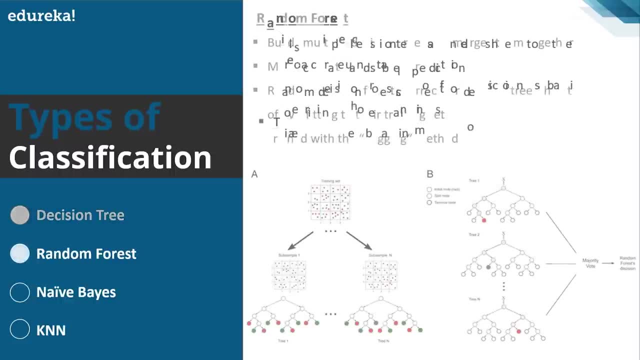 $25, then you'll just go and buy a hamburger, That's it All right. So this is about decision tree. Now, moving on ahead, Let's see What is a random forest. will random Forest build multiple decision trees and merges them together? 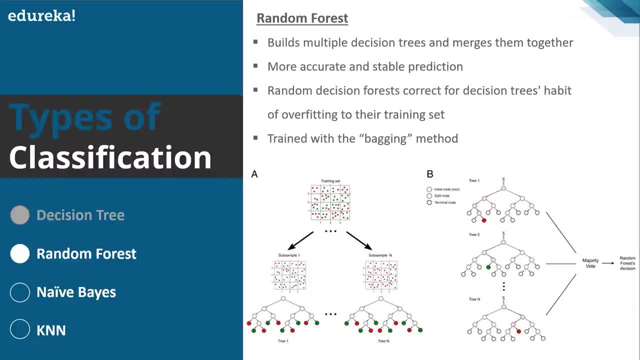 To get a more accurate and stable prediction. All right, most of the time, random Forest is trained with a bagging method. The bagging method is based on the idea that the combination of learning model increases the overall result. If you are combining the learning from different models and then 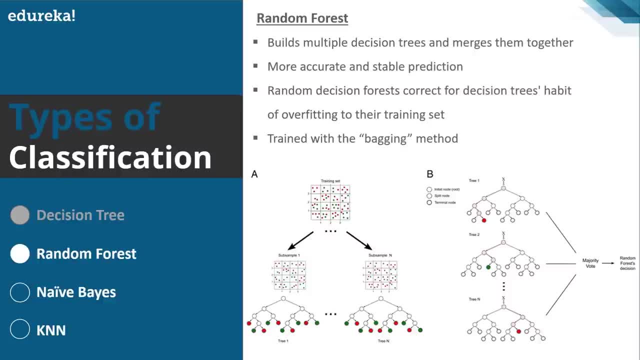 clubbing it together. what it will do? It will increase the overall result. Fine. Just one more thing: if the size of your data set is huge, then in that case one single decision tree would lead to a overfit model, Same way, Like a single person might have its own perspective on the complete population, as a population is. 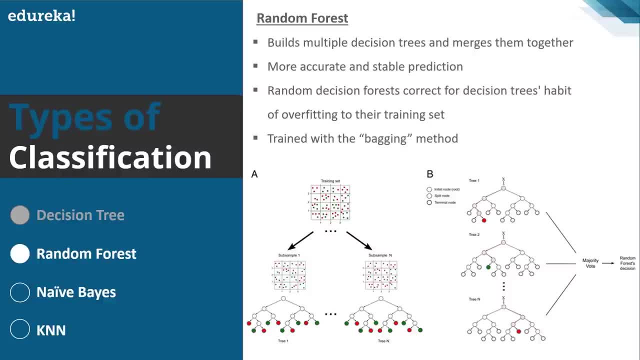 very huge right. However, if we implement the voting system and ask different individual to interpret the data, then we would be able to cover the pattern in a much meticulous way. Even from the diagram you can see that in section a we have a large training data set. What we do? we first divide our training. 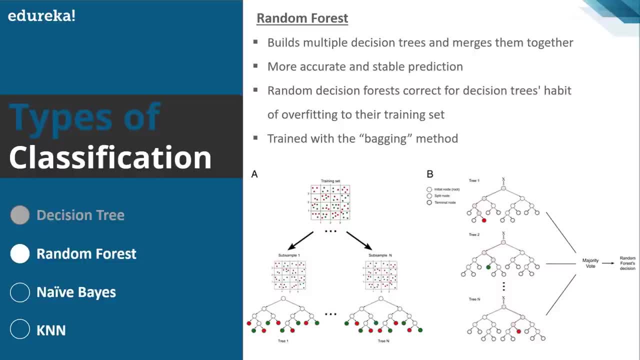 data set into n sub samples, All right, and we create a decision tree for each sub sample. Now, in the B part, what we do? we take the vote out of every decision made by every decision tree And finally we club the vote to get the random Forest decision. fine. 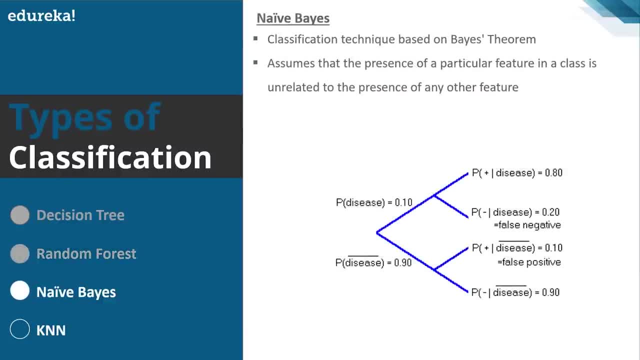 Let's move on ahead. Next we have nabias. So nabias is a classification technique which is based on Bayes theorem. It assumes that presence of any particular feature in a class is completely unrelated to the presence of any other feature. nabias is simple and easy to implement algorithm. 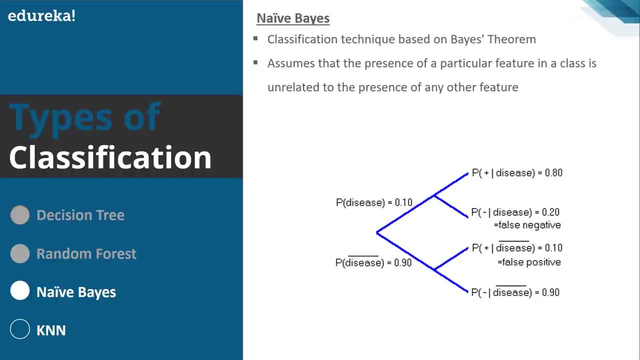 And due to a simplicity, this algorithm might outperform more complex model when the size of the data set is not large enough. All right, a classical use case of nabias is a document classification, and that what you do? you determine whether given text corresponds to one or more categories in the 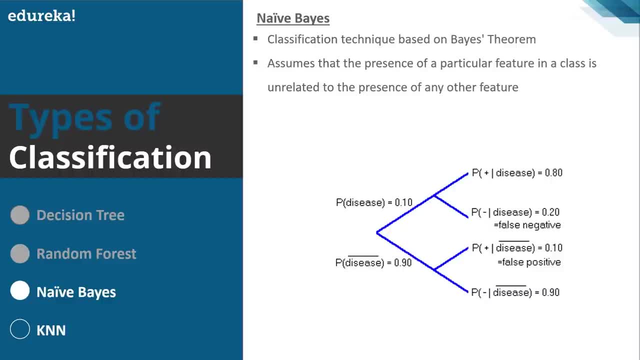 text case. the features used might be the presence or absence of any keyword. So this was about nabias. from the diagram You can see that using nabias, we have to decide whether we have a disease or not. First what we do, we check the probability of having a disease. 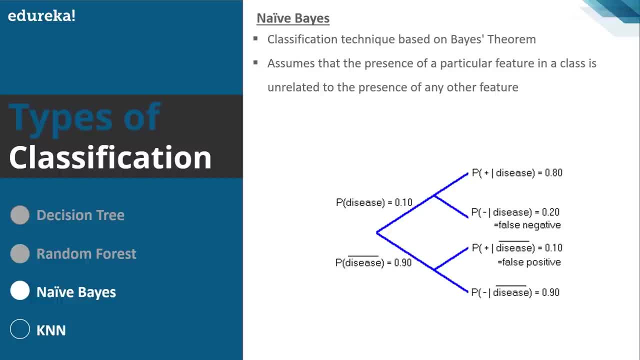 and not having the disease right. probability of having a disease is 0.1. While, on the other hand, probability of not having a disease is 0.9.. Okay, First let's see when we have disease and we go to doctor early. 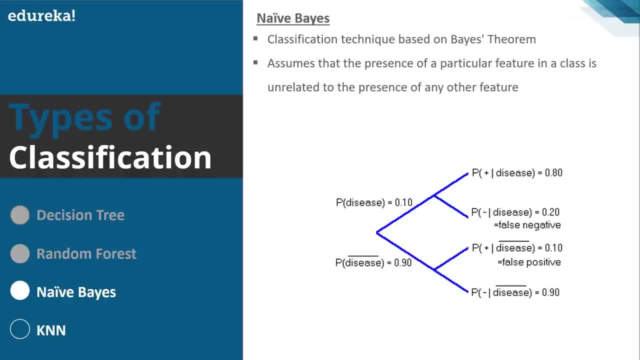 So when you visited the doctor and the test is positive, so probability of having a positive test when you're having a disease is 0.80 and probability of a negative test when you already have a disease That is 0.20.. This is also a false negative statement, as the test is detecting negative. 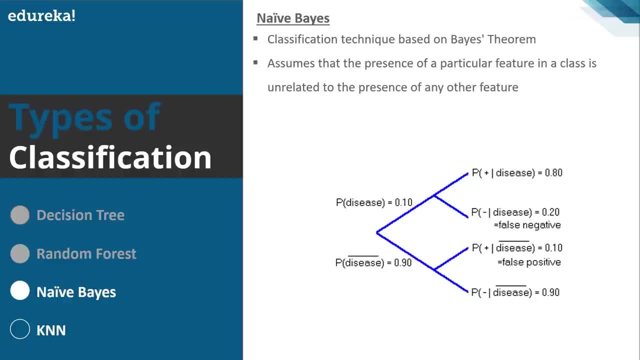 but you still have the disease right. So it's a false negative statement. Now let's move ahead when you don't have the disease at all. So probability of not having a disease is 0.9.. And when you visit the doctor and the doctor is like, yes, you have the disease. 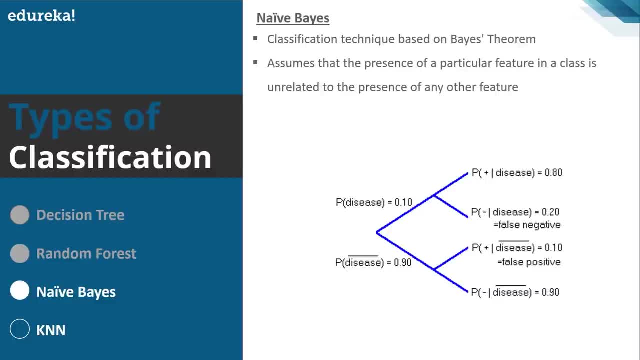 but you already know that you don't have the disease, So it's a false positive statement. So probability of having a disease when you actually know there is no disease is 0.1.. And probability of not having a disease when you actually know there is no disease. 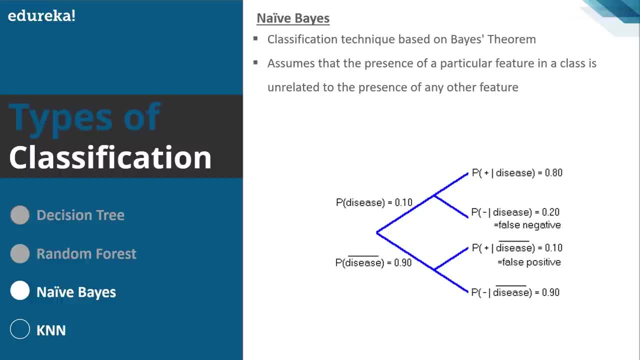 So and the probability of it is around 0.90.. Fine, It is same as probability of not having a disease in the test is showing the same result. It's a true positive statement, So it is 0.9.. All right, so let's move on ahead and discuss about KNN algorithm. 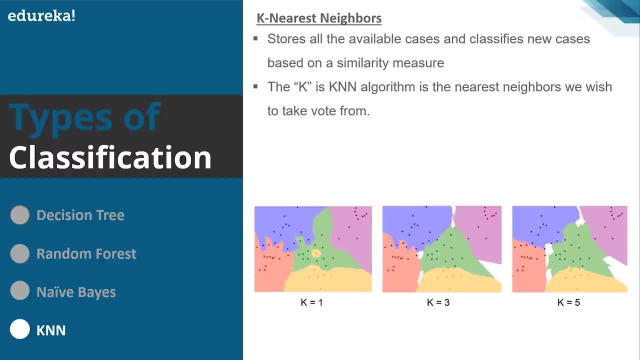 So this KNN algorithm or the K nearest neighbor. It stores all the available cases and classifies new cases based on The similarity measure. The K in the KNN algorithm is the nearest neighbor We wish to take vote from. for example, if K equal 1, then the object is simply assigned to the class of that single nearest neighbor from the diagram. 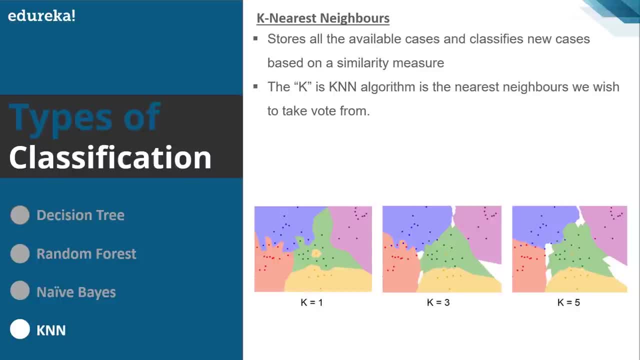 You can see the difference in the image when K equal 1, K equal 3 and K equal 5, right Well, the modern systems are now able to use the K nearest neighbor for visual pattern recognition to scan and detect hidden packages in the bottom bin of a shopping cart. 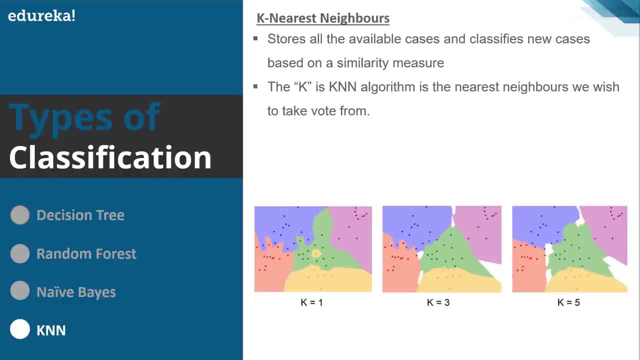 At the checkout. if an object is detected which matches exactly to the object listed in the database, then the price of the spotted product could even automatically be added to the customer's bill, While this automated billing practice is not used extensively at this time, but the technology has been developed and is available for use. 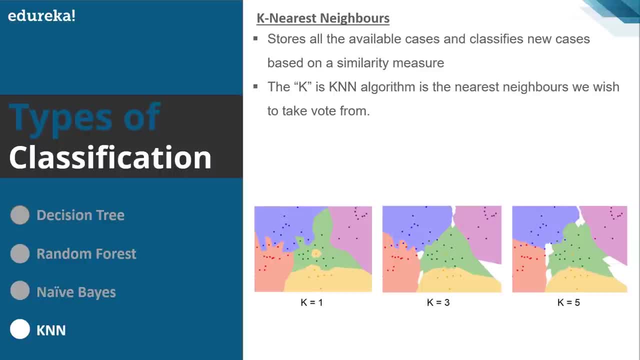 If you want, you can just use it and you have one more thing. K nearest neighbor is also used in retail to detect patterns in the credit card. uses many new transactions scrutinizing Software application. use KNN algorithms to analyze register data and spot unusual pattern that indicates suspicious activity. 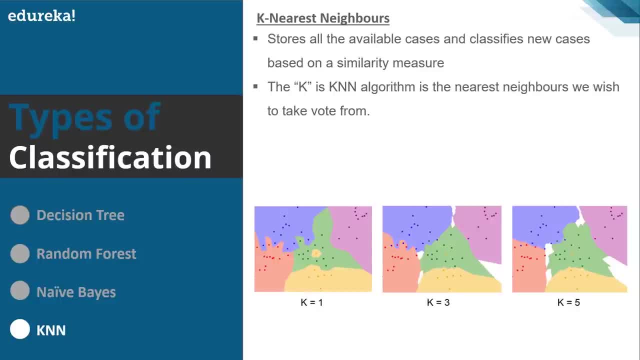 For example, if register data indicates that a lot of customers information is being entered manually rather than through automated scanning and swapping, then in that case this could indicate that the employees who are using the register are in fact stealing customers personal information. or for register data indicates that a particular good is being returned or exchanged multiple times. 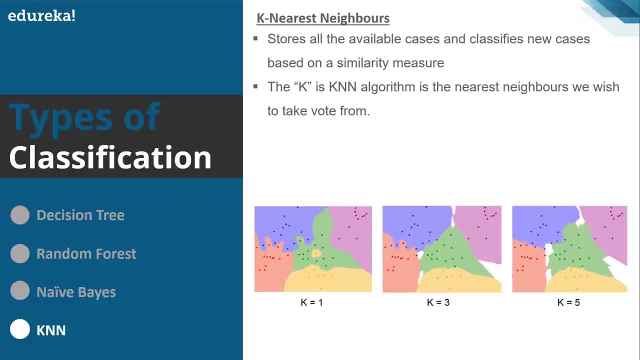 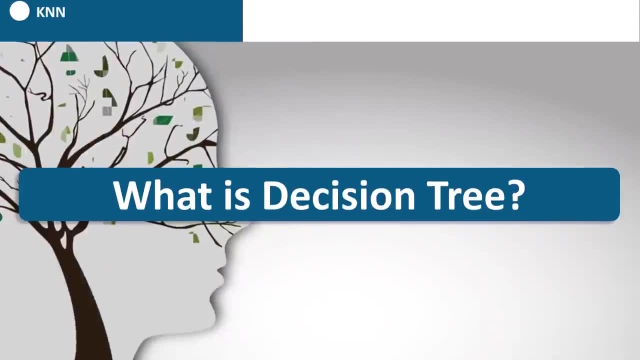 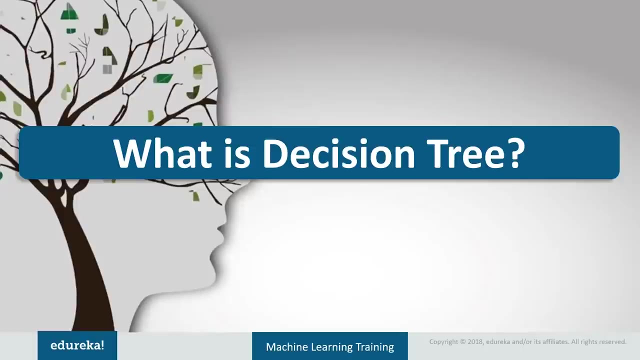 This could indicate that employees are misusing the return policy or trying to make money from doing the fake returns. right, So this was about KNN algorithm. fine, Since our main focus for this session will be on decision tree, So starting with, what is decision tree? but first let me tell you why did we choose decision tree to start with. 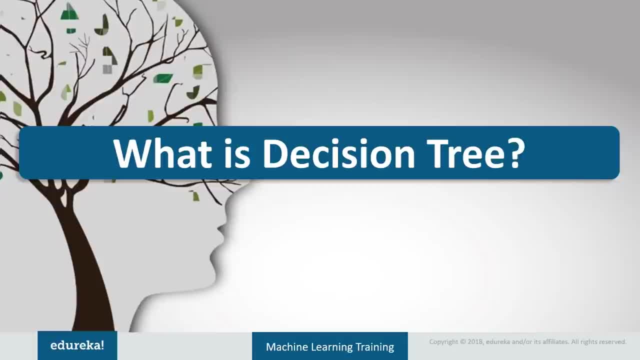 Well, these decision tree are really very easy to read and understand. It belongs to one of the few models that are interpretable where you can understand exactly why the classifier has made that particular decision right. Let me tell you a fact: that, for a given data set, 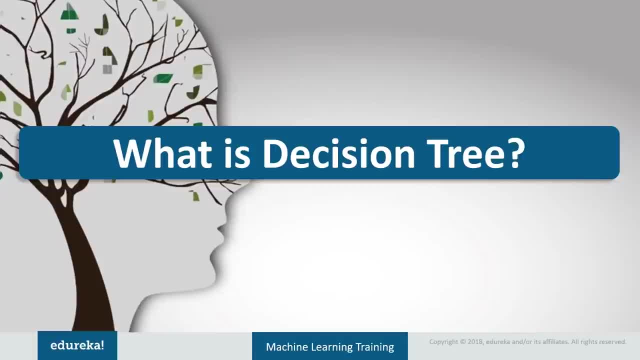 You cannot say that this algorithm performs better than that. It's like you cannot say that decision trees better than a bias or name biases performing better than decision tree. It depends on the data set right. You have to apply hidden trial method with all the algorithms one by one and then compare the result. 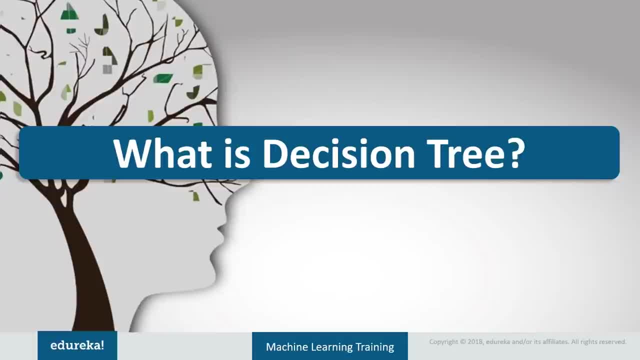 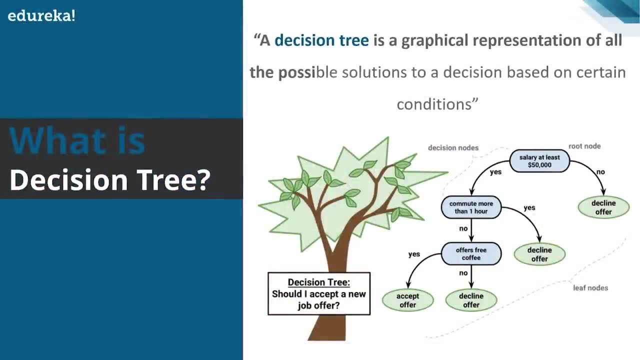 The model which gives the best result is the model which you can use It for better accuracy for your data set. All right, so let's start with what is decision tree? Well, a decision tree is a graphical representation of all the possible solution to a decision, based on certain conditions. 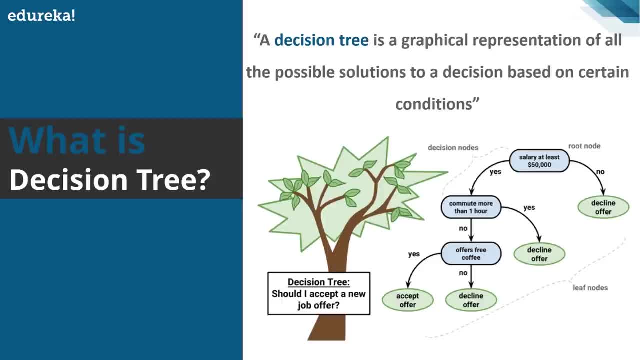 Now you might be wondering why this thing is called as decision tree. Well, it is called so because it starts with a root and then branches off to a number of solution, just like a tree, right? Even the tree starts from a root and it starts growing its branches. 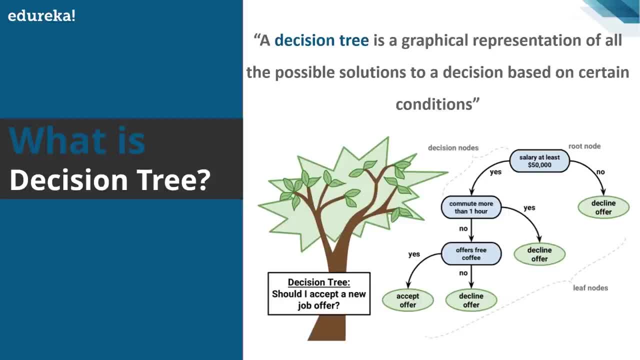 Once it gets bigger and bigger. similarly, in a decision tree, It has a rule which keeps on growing with increasing number of decision and the conditions. Now let me tell you a real life scenario. I won't say that all of you, but most of you, must have used it. 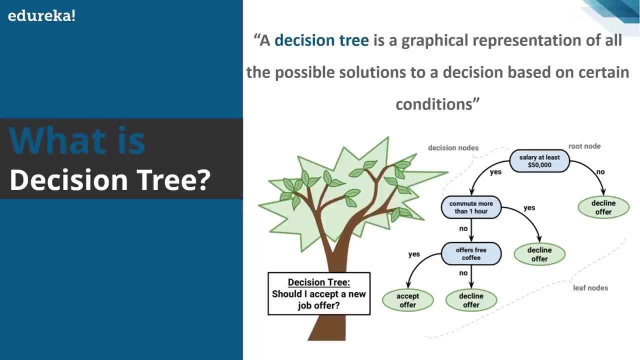 Remember, whenever you dial the toll-free number of your credit card company, it redirects you to his intelligent computerized assistant where it asks you questions like press 1 for English or press 2 for Hindi, press 3 for this, press 4 for that. right now. 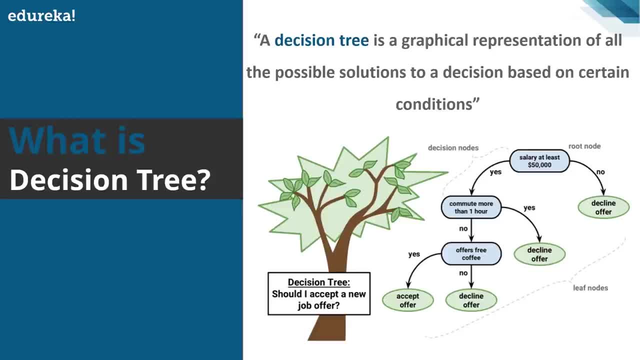 Once you select one, now again the tree directs you to a certain set of questions like press 1 for this, press 1 for that and similarly right. So this keeps on repeating until you finally get to the right person, right? you might think that you are caught in a voicemail hell. 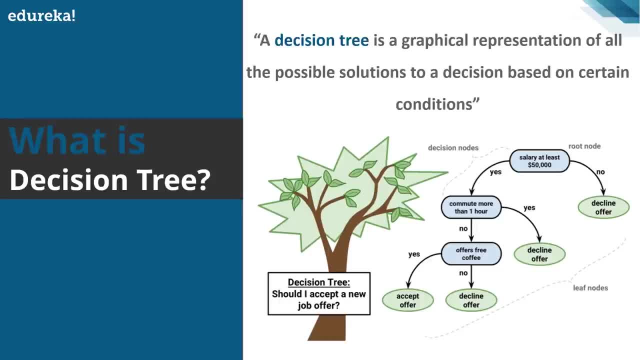 but what the company was actually doing. It was just using a decision tree to get you to the right person. All right, I'd like you to focus on this particular image for a moment. on this particular slide, You can see image where the task is: should I accept a new job offer or not? 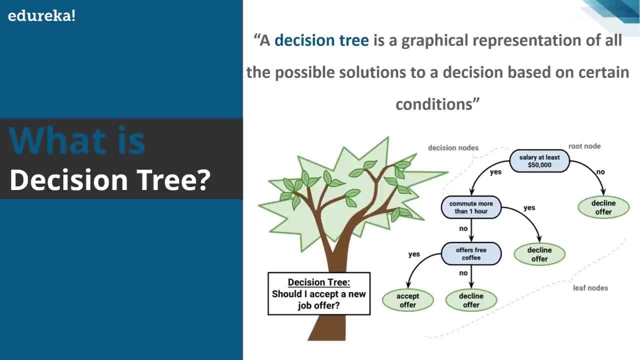 All right. so you have to decide that. for that, What you did, you created a decision tree. starting with the base condition, or the root node, was that the basic salary, or the minimum salary, should be $50,000.. If it is not $50,000,. then you are not at all accepting the offer a late. So if your salary is greater than $50,000, then you will further check whether the commute is more than one hour or not. If it is more than one hour, you will just decline the offer. if it is less than one hour: 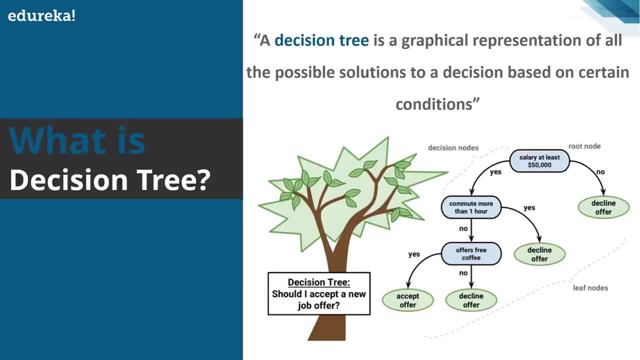 then you are getting closer to accepting the job offer. Then, further, what you'll do? you will check whether the company is offering free coffee or not. right, If the company is not offering the free coffee, then you will just decline the offer and have fit as offering the free coffee. 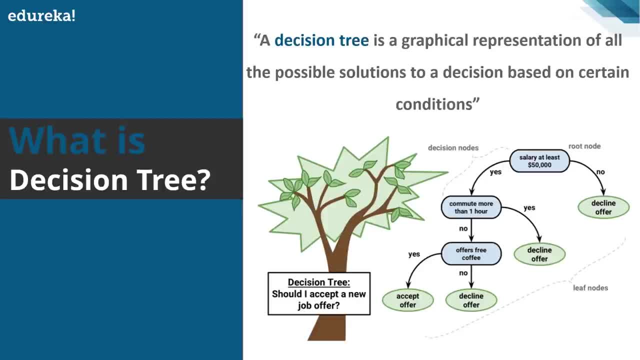 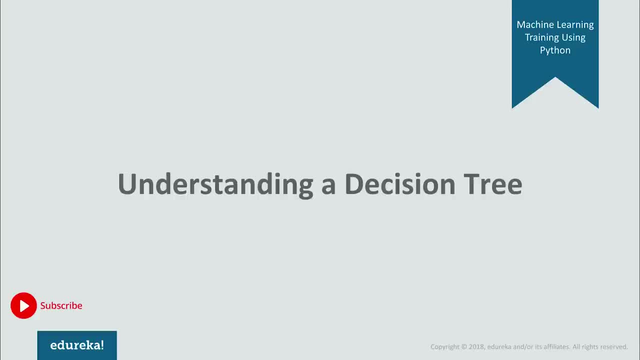 And, yeah, you will happily accept the offer, right? These are just our example of a decision tree. Now let's move ahead and understand a decision tree. Well, here is a sample data set that I'll be using it to explain you. 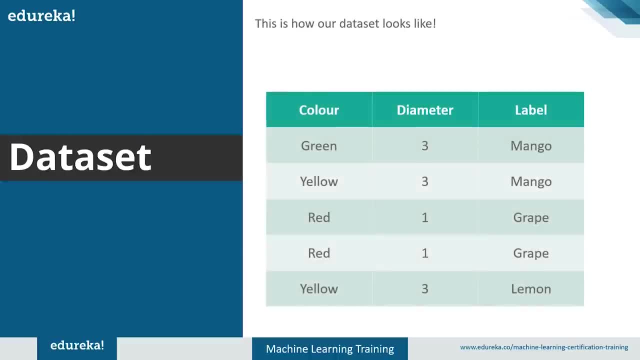 about the decision tree. All right, in this data set, each row is an example and the first two columns provide features or attributes. that describes the data and the last column gives the label or the class we want to predict and, if you like, you can just modify this data. 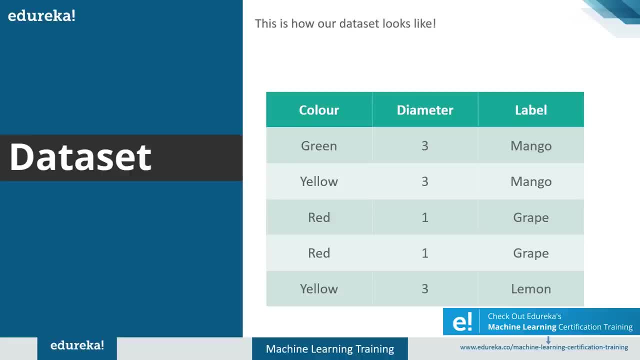 by adding additional features and more example, and our program will work in exactly the same way. fine, Now, this data set is pretty straightforward, except for one thing. I hope you have noticed that it is not perfectly separable. Let me tell you something more about that. as in the second, 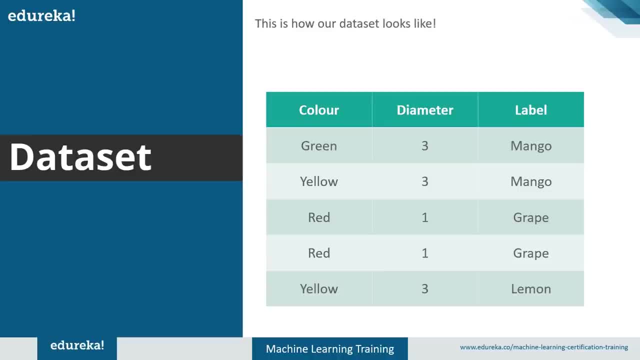 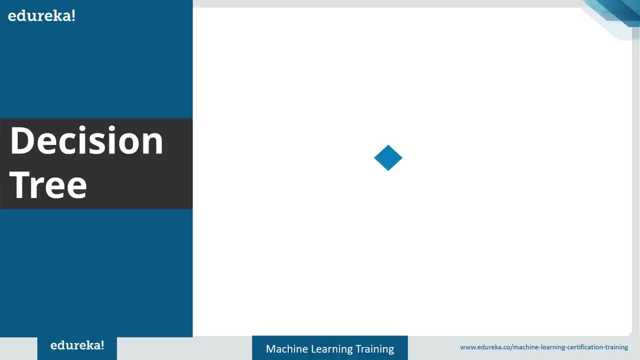 and fifth examples. they have the same feature, But different labels. both have yellow as their color and diameter as three, but the labels are mango and lemon. fine, Let's move on and see how our decision tree handles this case. All right, in order to build a tree, will use a decision tree algorithm. 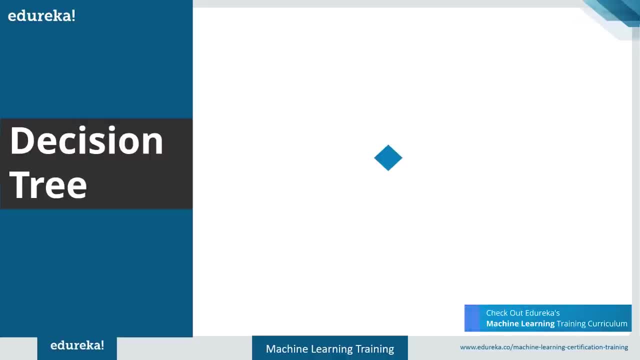 called cart. the Scott algorithm stands for classification and regression tree algorithm. All right, let's see a preview of how it works. All right, to begin with, we'll add a root node for the tree and all the nodes receive a list of rows as input, and the root will receive the entire training data set. 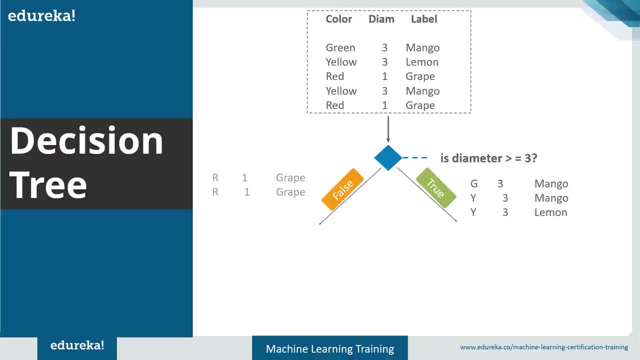 Now each node will ask- true and false- question about one of the feature and in response to that question, will split or partition the data set into two different subsets. These subsets then become input to child node. We are to the tree and the goal of the question is. 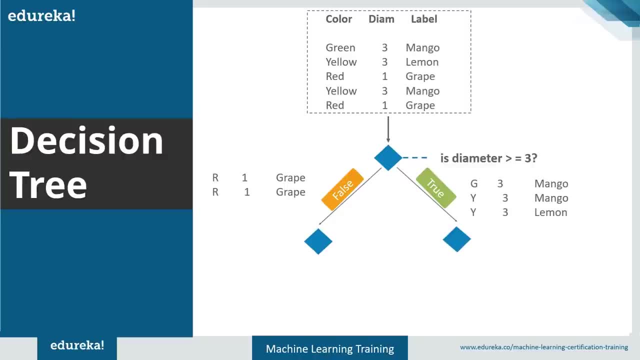 to finally unmix the labels as we proceed down, or in other words, to produce the purest possible distribution of the labels at each node. For example, the input of this node contains only one single type of label, So we could say that it's perfectly unmixed. 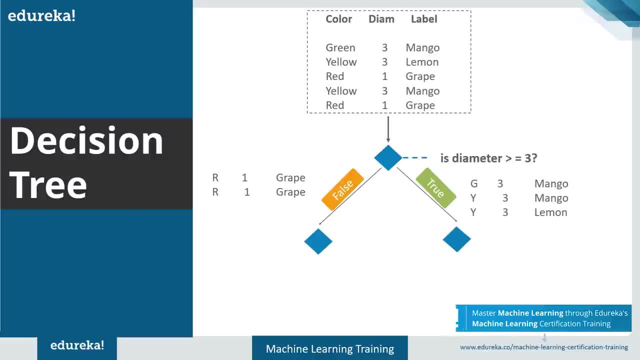 There is no uncertainty about the type of label, as it consists of only grapes right. on the other hand, the labels in this node are still mixed up, So we would ask another question to further drill it down. right, But before that we need to understand which question to ask. 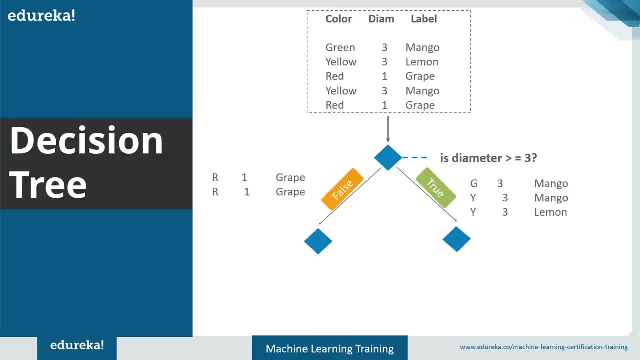 and when. and to do that we need to quantify how much question helps to unmix the label. and we can quantify the amount of uncertainty at a single node using a metric called Gini impurity. and we can quantify how much of question reduces that uncertainty using a concept called information game will. 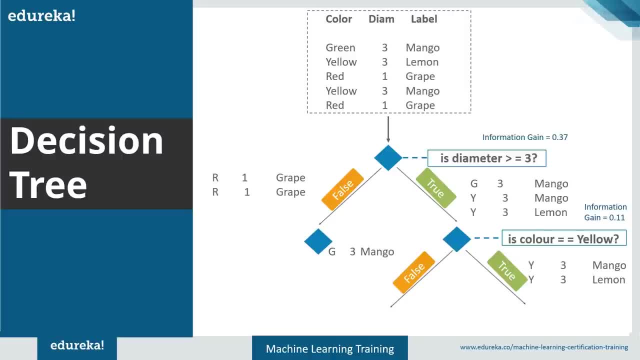 use these to select the best question to ask at each point, and then what we'll do will iterate the steps, will recursively build the tree on each of the new node, will continue dividing the data until there are no further question to ask and finally we reach to our leaf. 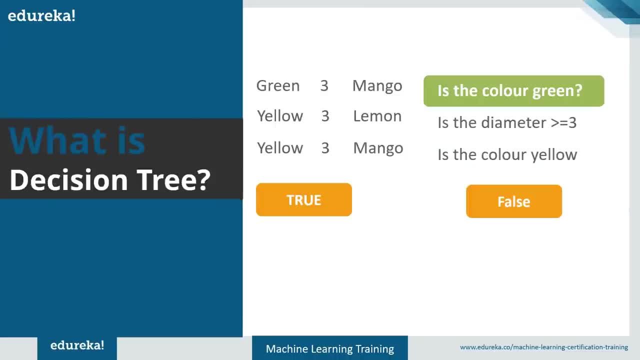 All right, All right, So this was about decision tree. So, in order to create a decision tree, first of all, what you have to do, you have to identify different set of questions that you can ask to a tree, like: is this color green and what will be these question? these questions will: 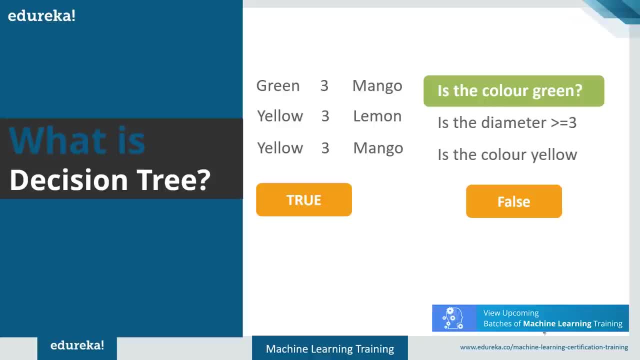 be decided by your data set, like: is this colored green? is the diameter greater than equal to 3? is the color yellow right questions resembles to your data set. Remember that, All right. So if my color is green, then what it will do? it will divide. 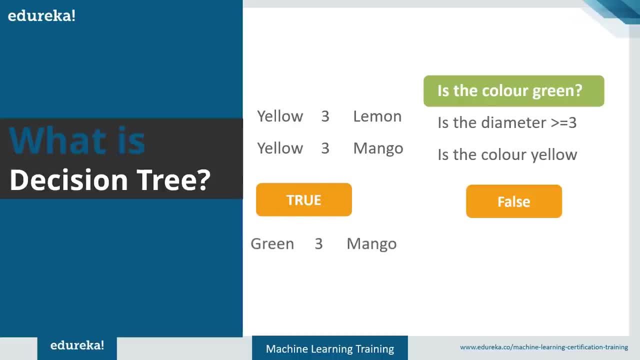 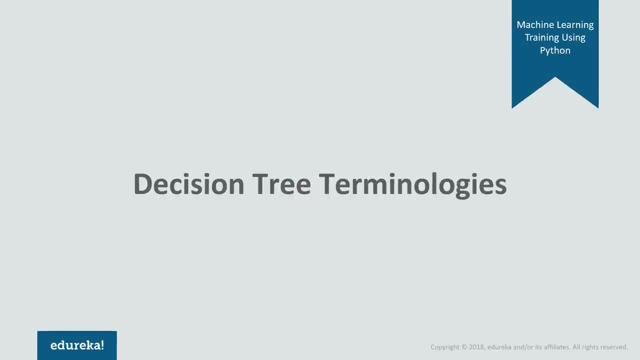 into two part. first the green mango will be in the true, while on the false We have lemon and the map all it if the color is green or the diameter is greater than equal to 3 or the color is yellow. Now let's move on and understand about decision tree terminologies. 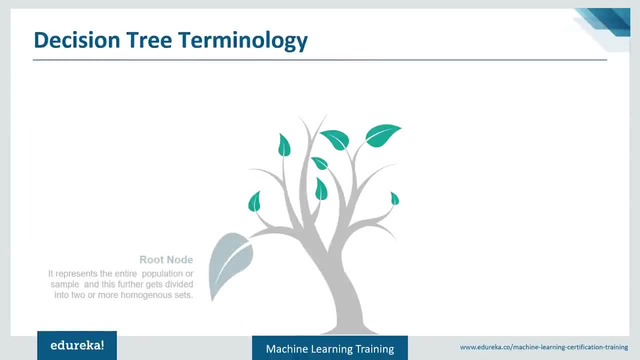 All right. So, starting with root node, root node is the base node of a tree. The entire tree starts from a root node. In other words, it is the first node of a tree. It represents the entire population or sample, and this entire population. 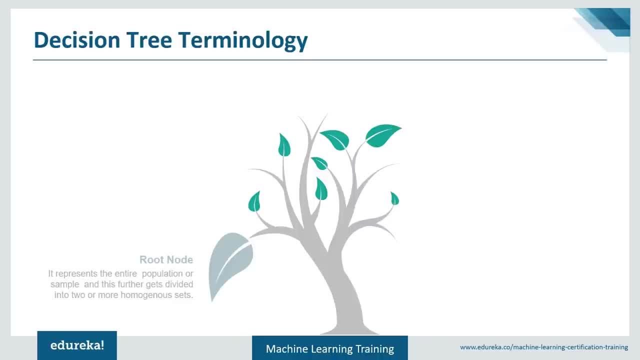 Is further segregated or divided into two or more homogeneous set, fine. Next is the leaf node. Well, leaf node is the one when you reach at the end of the tree, right That is. you cannot further segregated down to any other level. That is the leaf node. 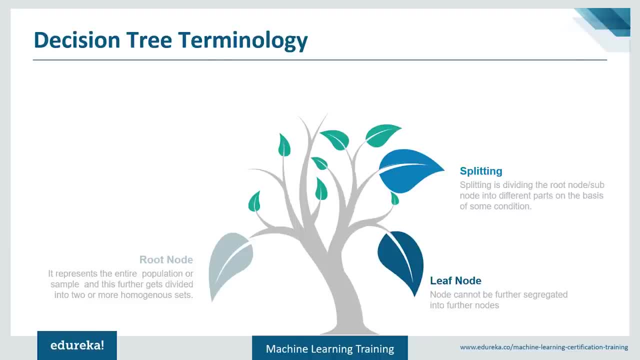 Next is splitting. splitting is dividing your root node or your node into different sub part on the basis of some condition. All right, then comes the branch or the sub tree. Well, this branch or sub tree gets formed When you split the tree, suppose, when you split a root node. 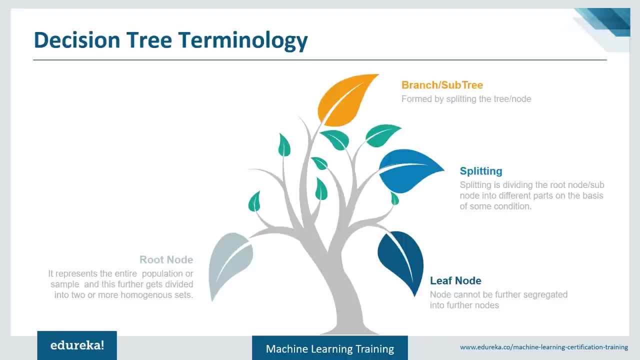 it gets divided into two branches or two sub trees, right. Next is the concept of pruning. Well, you can say that pruning is just opposite of splitting. what we are doing here. We are just removing the sub node of a decision tree. We'll see more about pruning later in this session. 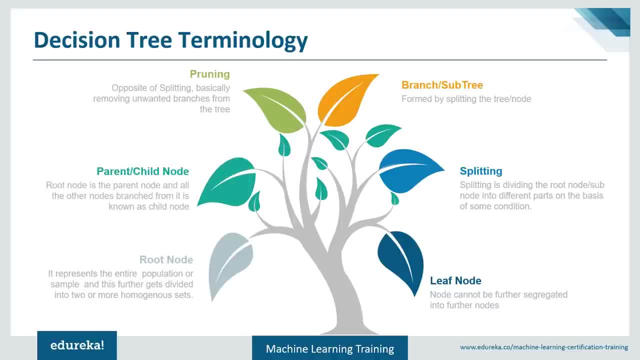 All right, let's move on ahead. Next is parent or child node. Well, first of all, root node is always the parent node and all other nodes associated with that is known as child node. Well, you can understand it in a way that all the top node 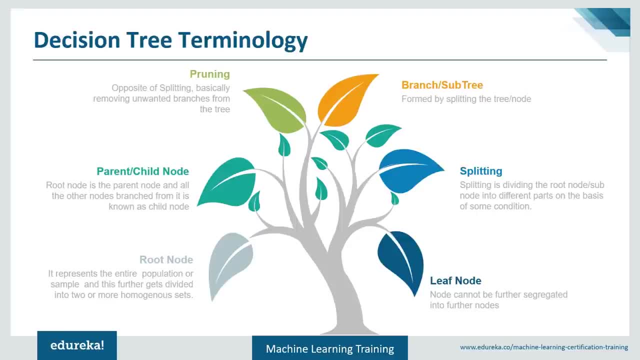 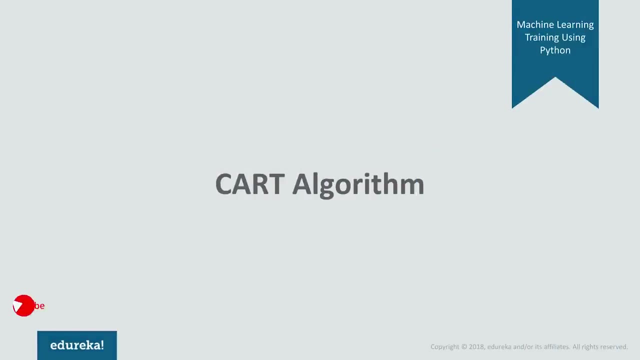 belongs to a parent node and all the bottom node which are derived from a top node is a child node. The node producing a further node is a child node and the node which is producing it is a parent node. simple concept, right? Let's use the cart algorithm and design a tree manually. 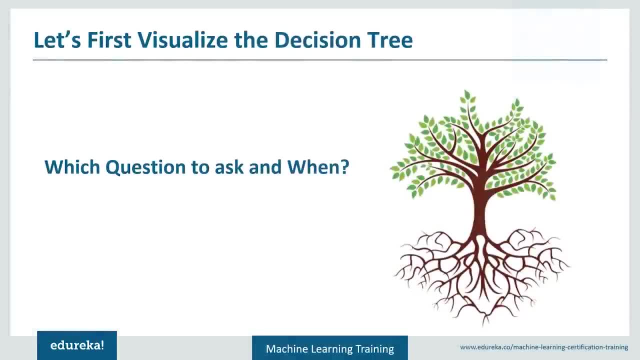 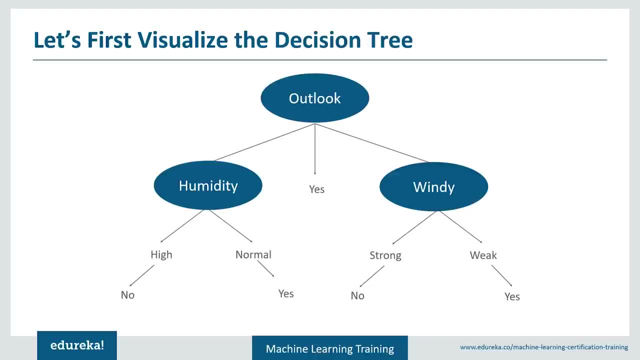 So, first of all, what do you do? You decide which question to ask and when. so how will you do that? So let's first of all visualize the decision trees. So there's the decision tree which will be creating manually, All right. 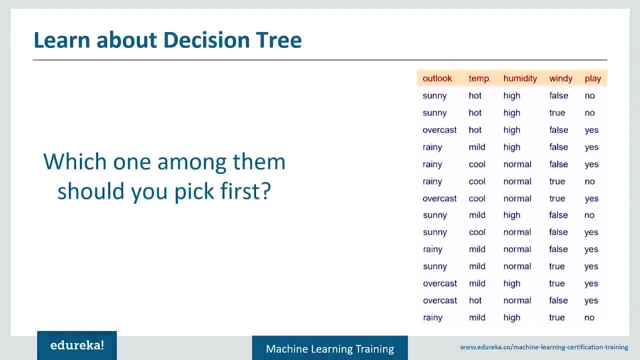 First of all, let's have a look at the data set. You have Outlook, temperature, humidity and windy as your different attribute. on the basis of that, You have to predict that, whether you can play or not. So which one among them should you pick first? answer determine. 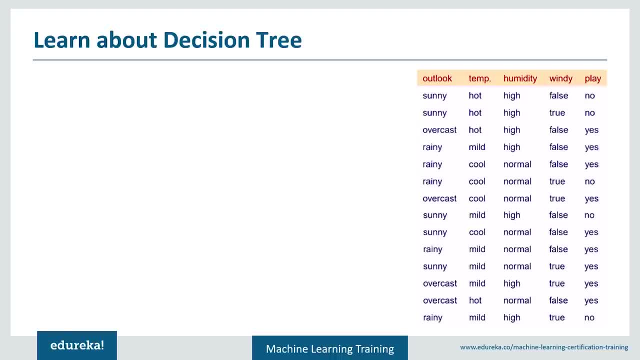 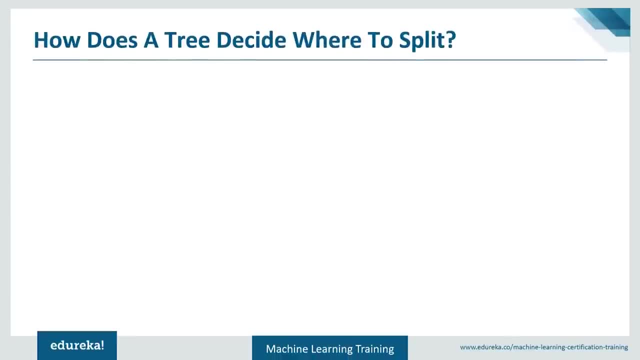 the best attribute that classifies the training data. All right, So how will you choose the best attribute? or how does a tree decide where to split? or how the tree will decide its root node will. before we move on and split a tree, There are some terminologies that you should know. 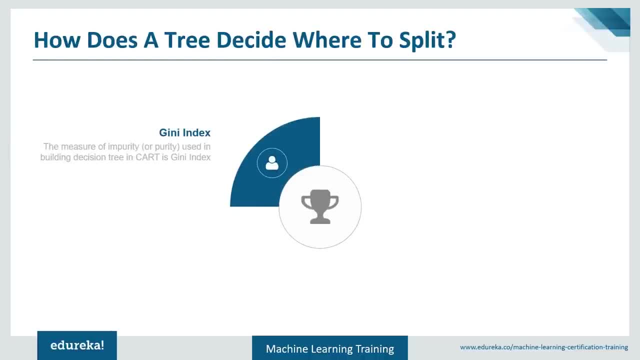 All right, first being the genie index. So what is this genie index? This genie index is the measure of impurity or purity used in building a decision tree in cart algorithm. All right, Next is information gain. This information gain is the decrease in entropy. 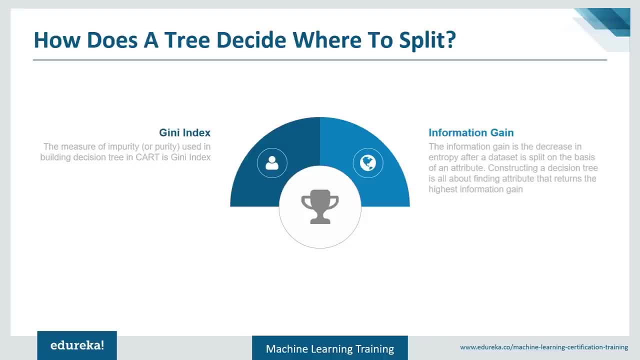 after data set is split on the basis of an attribute. constructing a decision tree is all about finding a attribute that returns The highest information gain. All right, so you'll be selecting the node that would give you the highest information gain, All right. 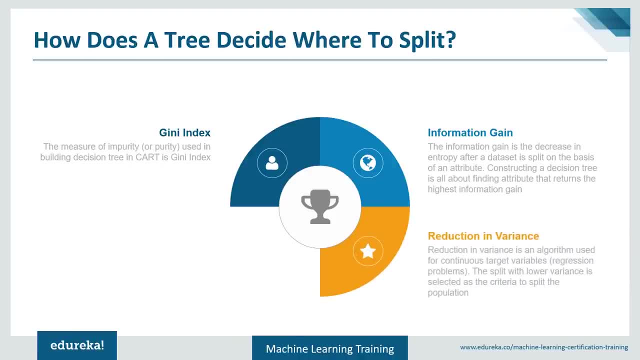 Next is reduction in variance. This reduction in variance is an algorithm which is used for continuous target variable or regression problems. The split with lower variance is selected as a criteria to split the population. see in general term, What do you mean by variance? variance is: 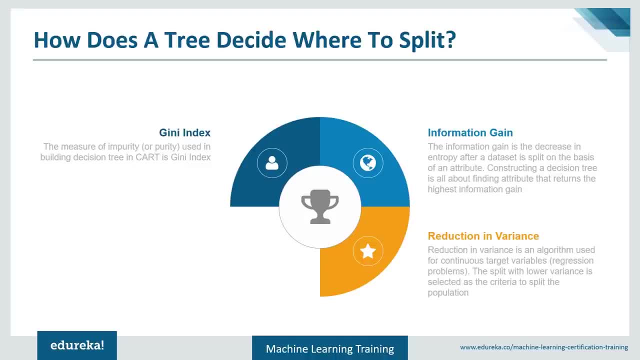 how much your data is wearing right. So if your data is less impure or it is more pure than in that case, the variation would be less, as all the data almost similar right. So there's also a way of splitting a tree that split. 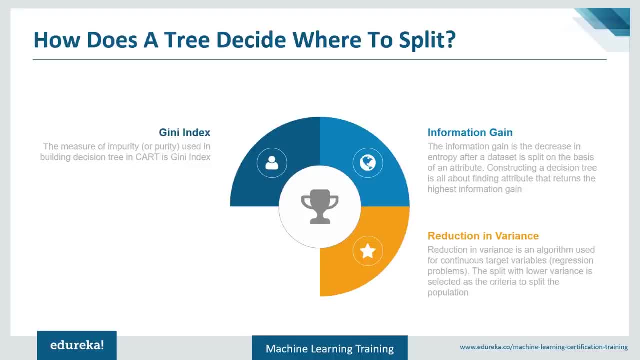 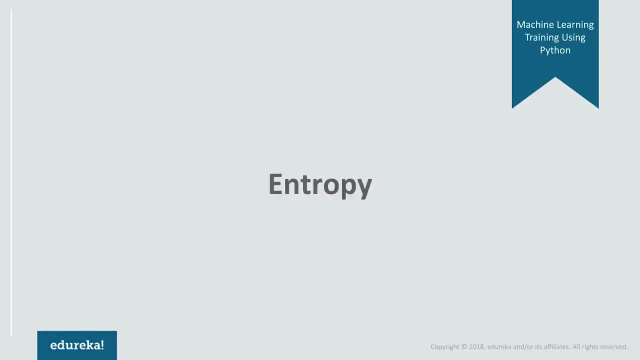 with lower variance is selected as a criteria to split the population. All right. Next is the chi-square. chi-square: It is an algorithm which is used to find out the statistical significance between the differences between sub nodes and the parent nodes. Fine, Let's move ahead. 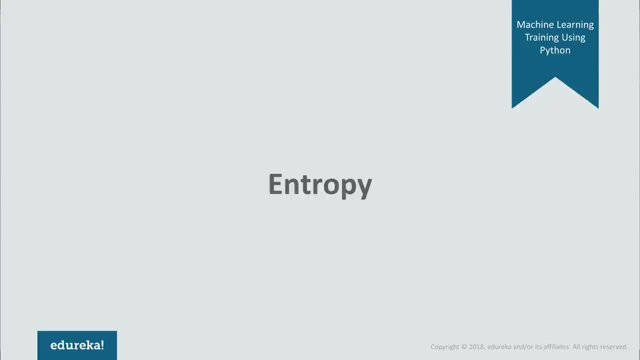 Now the main question is: how will you decide the best attribute? for now, Just understand that you need to calculate something known as information gain. the attribute with the highest information gain is considered the best. Yeah, I know your next question might be like: what is this information gain? 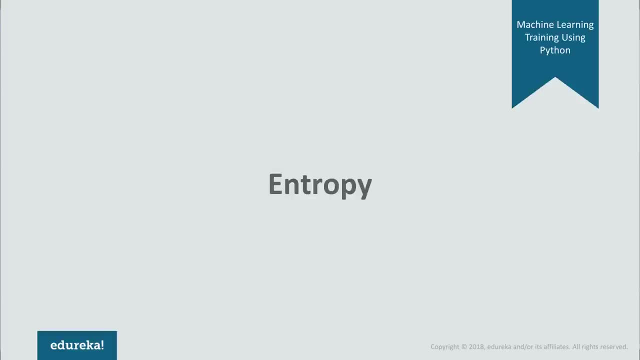 But before we move on and see what exactly information gain is, let me first introduce you to a term called entropy, because this term will be used in calculating the information gain. Well, entropy is just a metric which measures the impurity of something, or in other words, 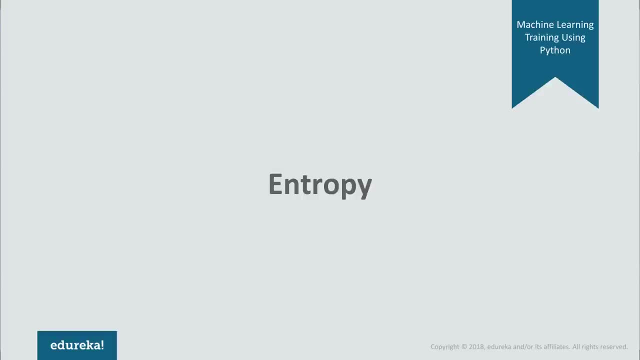 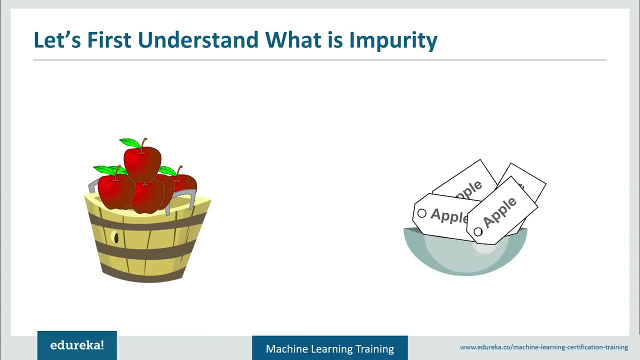 you can say that it's the first step to do before you solve the problem of a decision tree, As I mentioned here something about impurity. So let's move on and understand what is impurity. suppose you have a basket full of apples and another bowl. 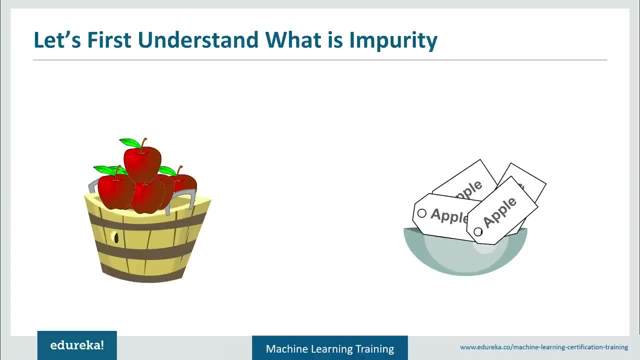 which is full of same label which says Apple. Now, if you are asked to pick one item from each basket and ball, then the probability of getting the apple and its correct label is one. So in this case you can say that impurity is zero. 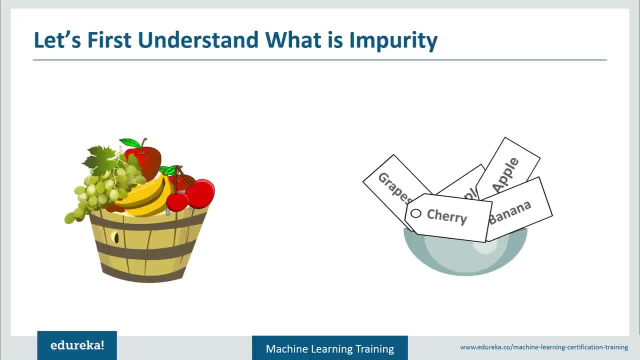 All right, Now what if there are four different fruits in the basket and four different labels in the ball? then the probability of matching the fruit to a label is obviously not one. It's something less than that. Well, it could be possible that I pick banana from the basket. 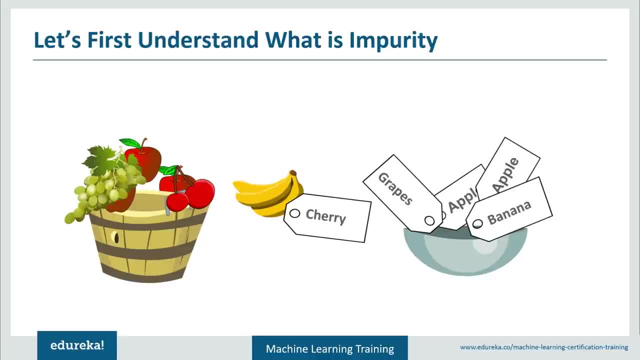 and when I randomly pick the label from the ball, it says a cherry. any random permutation and combination can be possible. So in this case I would say that impurities is nonzero. I hope the concept of impurity is clear. So, coming back to entropy, as I said, entropy is the measure. 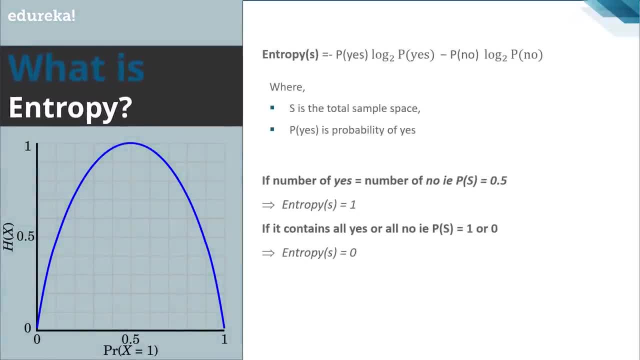 of impurity. from the graph on your left, You can see that, as the probability is 0 or 1, that is, either they are highly impure or they are highly pure- then in that case the value of entropy is 0 and when the probability is 0.5,. 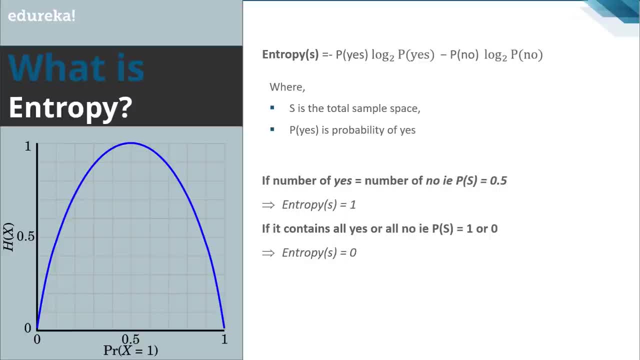 then the value of entropy is maximum. Well, what is impurity? impurity is the degree of randomness, how random a data is. So if the data is completely pure, in that case the randomness equals 0. or if the data is completely impure, 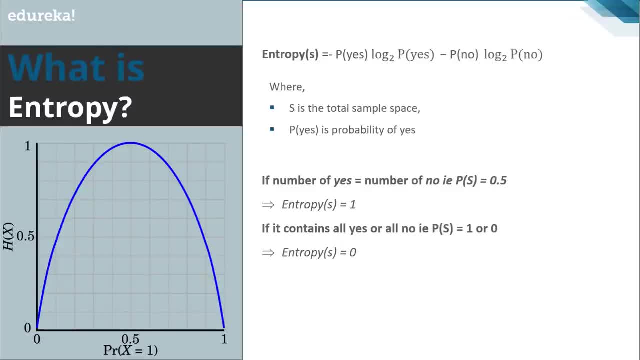 even in that case, the value of impurity will be 0. question Like why is it that the value of entropy is maximum at 0.5? might arise in your mind right. So let me discuss about that. Let me derive it mathematically, as you can see here on the slide. 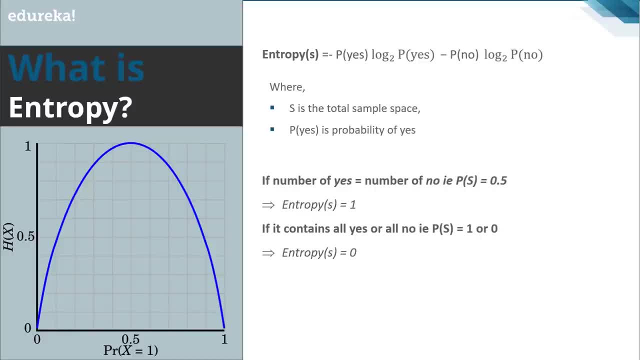 the mathematical formula of entropy is minus of probability of yes. Let's move on and see what this graph has to say mathematically. suppose s is our total sample space and it's divided into two parts- Yes and no, like in our data set. the result for playing was: 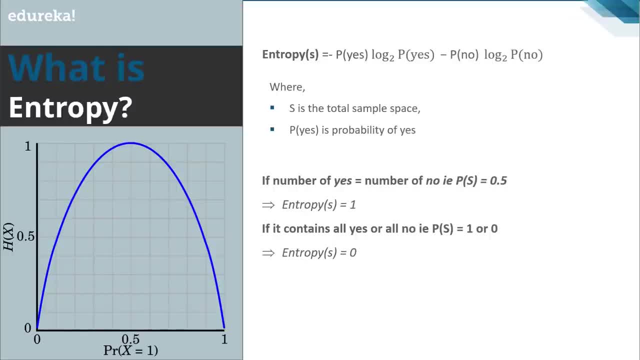 divided into two parts, either yes or no, which we have to predict. either we have to play or not, right? So for that particular case, you can define the formula of entropy as entropy of total sample space equals negative of probability of yes multiplied by log of probability of yes, with a base 2 minus probability. 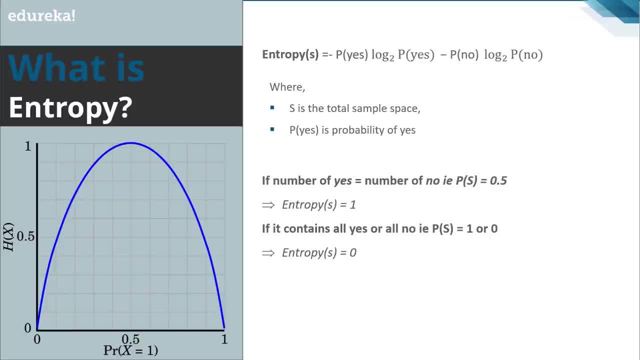 of no multiplied by log of probability of no, with base 2, where s is your total sample space and P of yes is the probability of yes and P of no is the probability of no. well, if the number of yes equal number of no, that is probability. 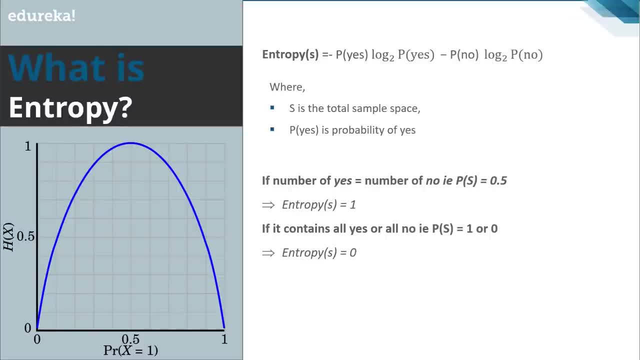 of s equals 0.5.. Right, since you have equal number of yes and no. so in that case, value of entropy will be one. just put the value over there. All right, let me just move to the next slide. I'll show you this. 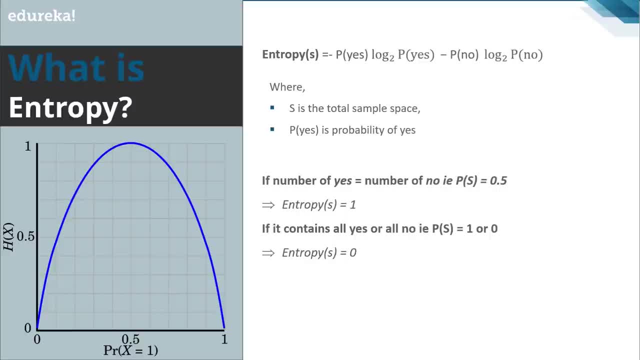 All right. Next is if it contains all yes or all no, that is, probability of a sample space is either 1 or 0, then in that case entropy will be equal to 0.. Let's see it mathematically: 1 by 1.. 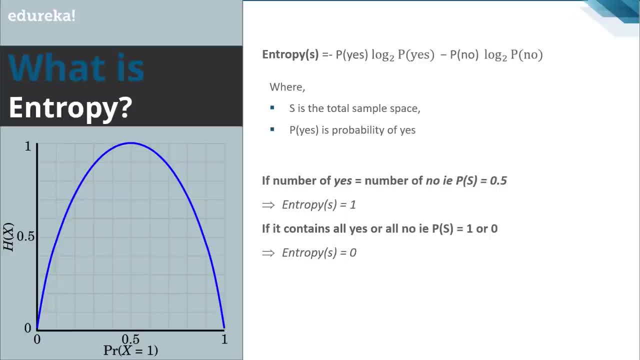 So let's start with the first condition where the probability was 0.5.. So this is our formula For entropy, right? So this is our first case right which we discuss, that when the probability of yes equal probability of no, that is in our data set. 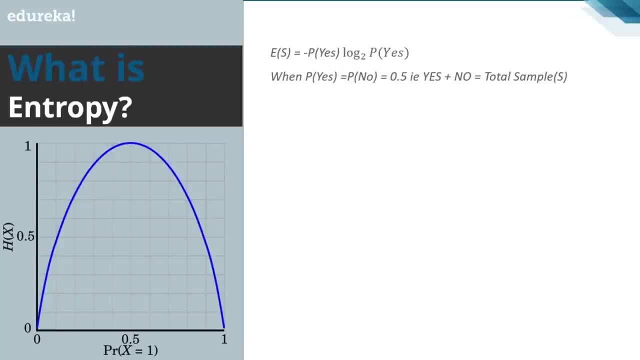 We have equal number of yes and no, All right, so probability of yes equal probability of no, and that equals 0.5. or in other words, you can say that yes plus no equal to total sample space. All right, since the probability is 0.5.. 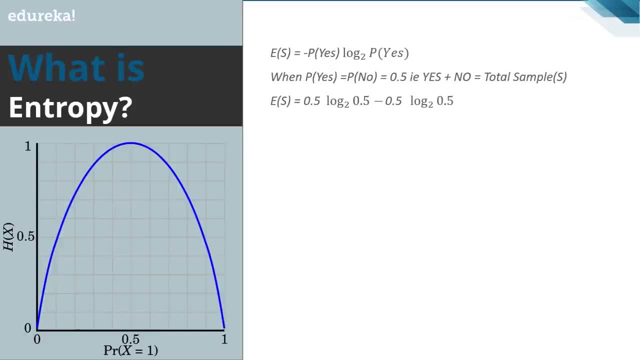 So when you put the values in the formula, you get something like this, and when you calculate it, You'll get the entropy of the total sample space as well. All right, let's see for the next case. What was the next case? either, you have total, yes, 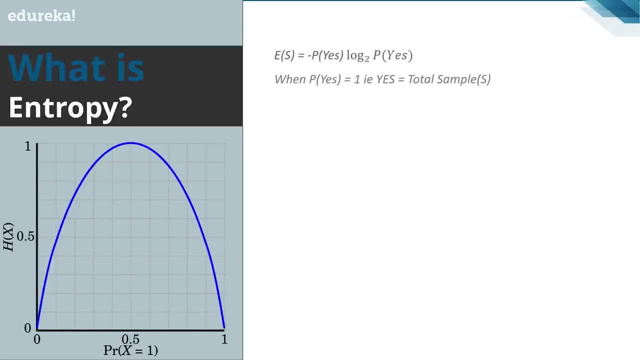 or you have total no. So if you have total yes, let's see the formula. when we have total yes, so you have all yes and 0, no fine. So probability of yes equal 1 and yes as the total sample space obviously. so in the formula when you put that thing up, you'll. 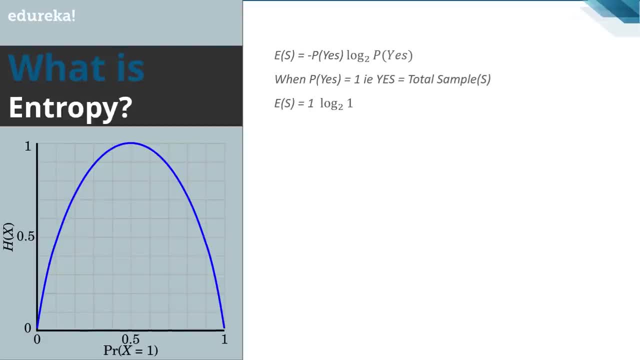 get entropy of sample space equal negative times of 1 multiplied by log of 1, as the value of log 1 equals 0. So the total thing will result to 0. similarly is the case with no. even in that case you'll get the entropy of total sample space as 0.. 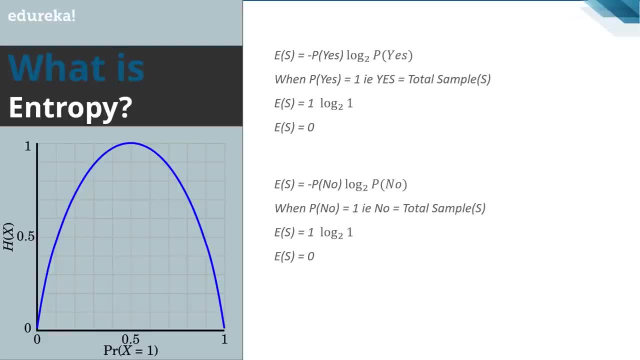 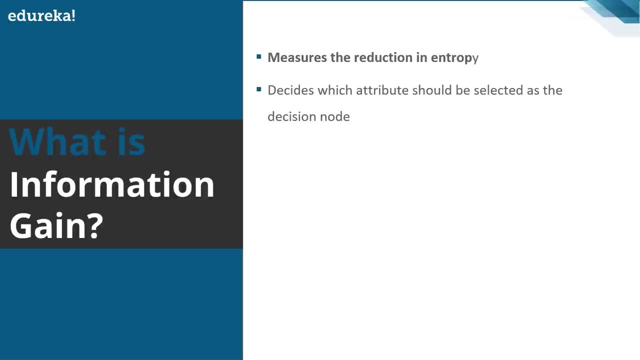 So this was all about entropy, All right. Next is: what is information gain? Well, information gain what it does. it measures the reduction in entropy. it decides which attribute should be selected as the decision node. if s is our total collection, then information gain equals entropy. 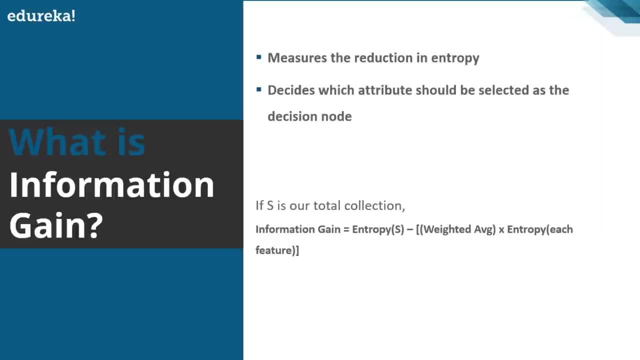 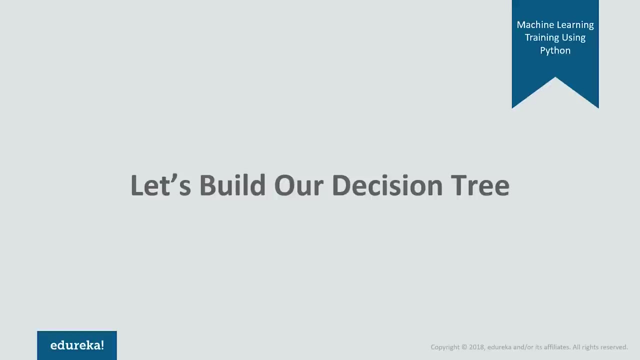 which we calculated just now, that minus weighted average multiplied by entropy of each feature. don't worry, We'll just see how to calculate it with an example. All right, So let's manually build a decision tree for our data set. So there's our data set, which consists of 14 different. 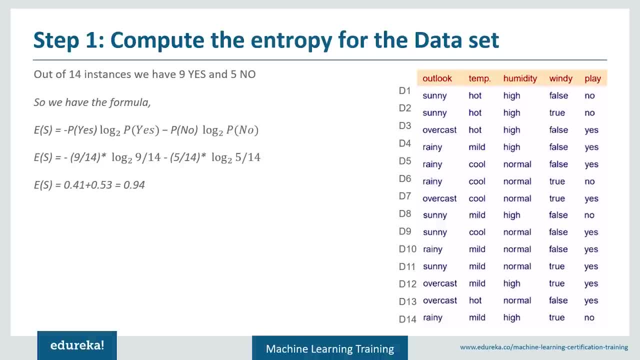 instances, out of which we have nine Yes and five No. all right, So we have the formula for entropy, just put over that, since nine years. So total probability of yes equals 9 by 14 and total probability of no equals 5 by 14.. 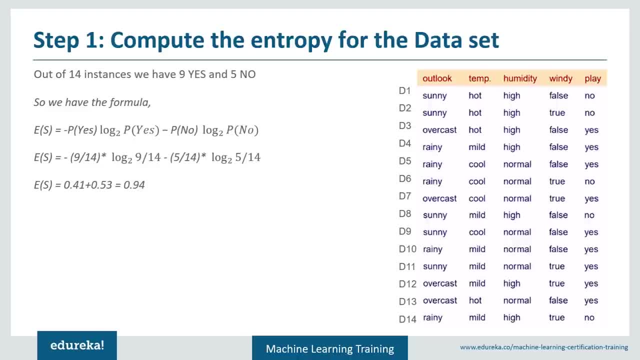 And when you put up the value and calculate the result, you will get the value of entropy as 0.94.. All right, So this was your first step, that is, compute the entropy for the entire data set. All right, Now you have to select that out of Outlook: temperature, humidity. 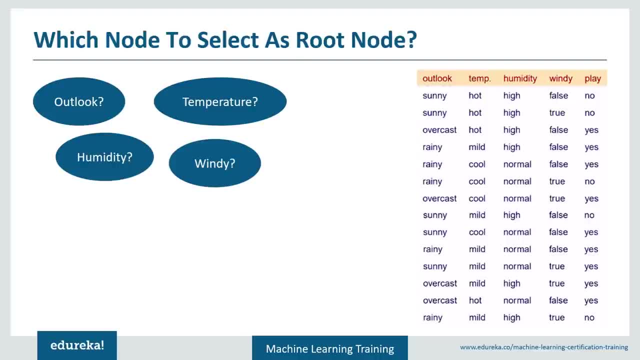 and windy. which of the node should you select as the root node? big question, right? How will you decide that this particular node should be chosen at the base node, and on the base of that only I'll be creating the entire tree? how you'll select that? 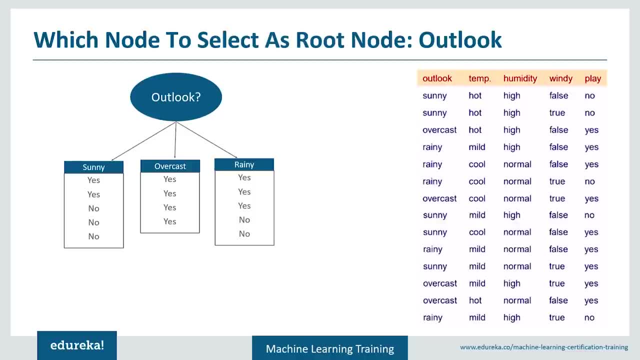 Let's see. So you have to do it one by one. you have to calculate the entropy and information gain for all of the different nodes, So starting with Outlook. so Outlook has three different parameters: sunny, overcast and rainy. So first of all, select how many number of yes. 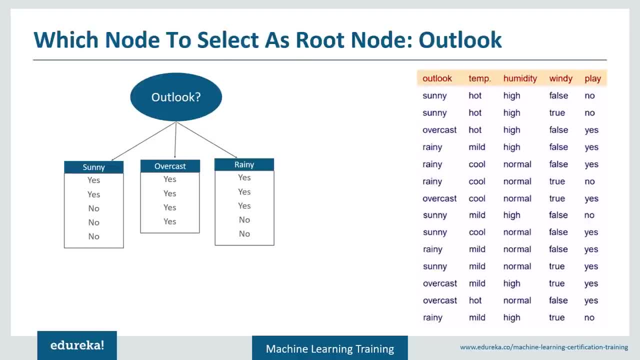 and no are there in the case of Sunny, like when it is Sunny, how many number of yes and how many number of no's are there? So in total, we have two years and three knows. in case of Sunny, in case of overcast, we have all yes. 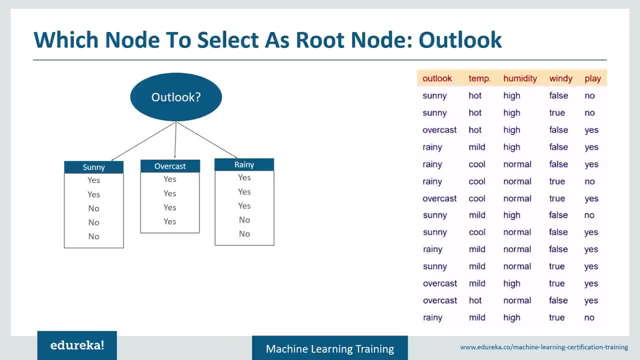 So if it is overcast, then we'll surely go to play. It's like that, All right. and next it is rainy, then total number of years equal 3 and total number of no equals to fine. Next, what we do? we calculate the entropy for each feature. 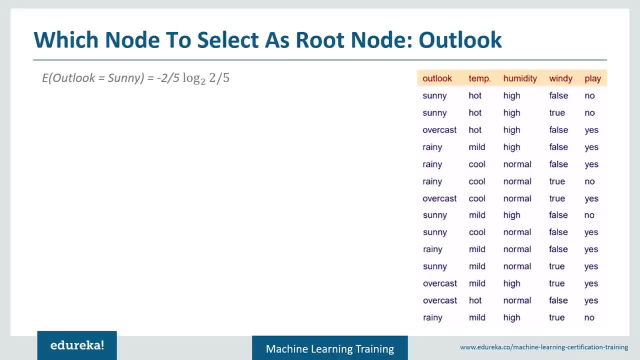 for here We are calculating the entropy when Outlook equals Sunny. first of all, we are assuming that Outlook is our root node and for that we are calculating the information gain for it. All right. So in order to calculate the information gain, remember the formula: it was entropy of the total sample space. 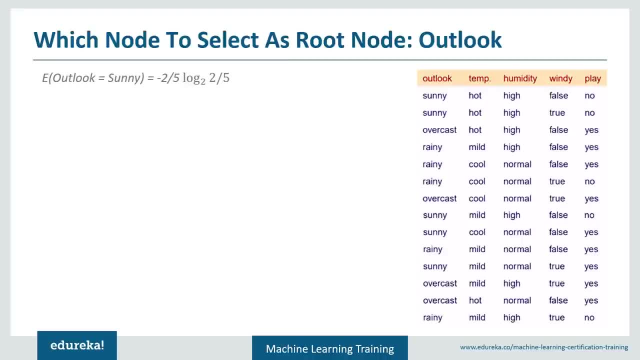 minus weighted average multiplied by entropy of each feature. All right, So what we are doing here? we are calculating the entropy of Outlook when it was Sunny. So total number of years when it was Sunny was 2 and total number of no that was 3. fine, 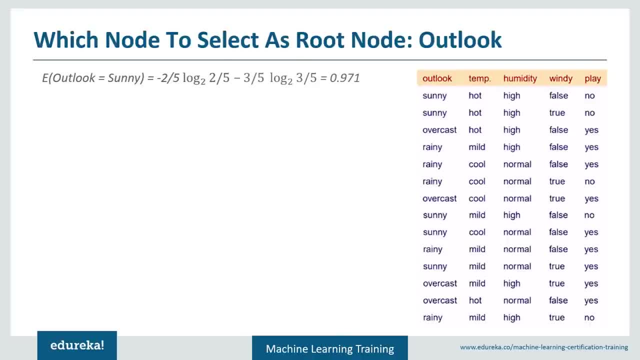 So let's put up in the formula, since the probability of yes is 2 by 5 and the probability of no is 3 by 5.. So you will get something like this. All right, so you are getting the entropy of Sunny as 0.971. fine. 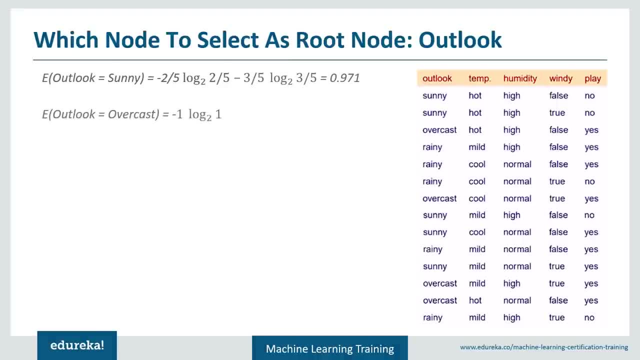 Next, you'll calculate the entropy for overcast. when it was overcast, remember, it was all yes, right? So the probability of yes equal 1 and when you put over that you'll get the value of entropy as 0. fine, And when it was rainy: rainy has 3s and 2 nose. 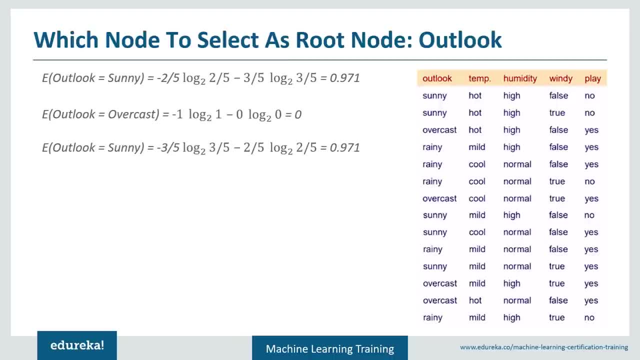 So probability of yes in case of Sunny is 3 by 5 and probability of no in case of Sunny is 2 by 5, and when you add the value of probability of yes and probability of no to the formula, you get the entropy of Sunny as 0.971. fine, 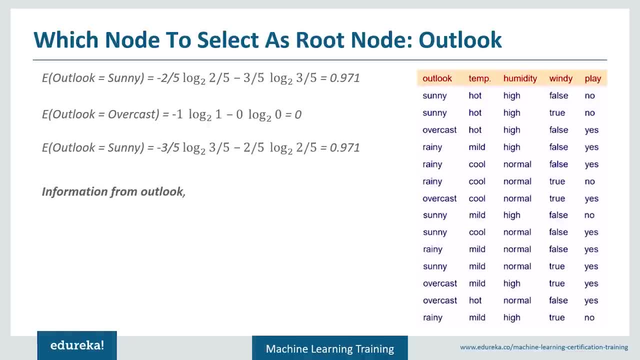 Now you have to calculate how much information you're getting from Outlook. that equals weighted average. All right. So what was this weighted average? total number of years and total number of? no fine, So information from Outlook equals 5 by 14. from where does this? 5 came over. 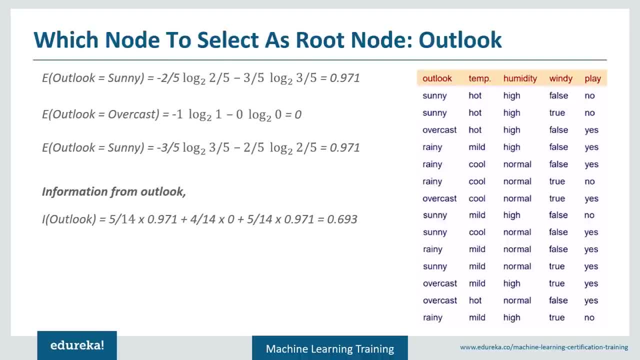 We are calculating the total number of sample space within that particular Outlook. when it was Sunny, right? So in case of Sunny there was two years and three, knows all right. So weighted average for Sunny would be equal to 5 by 14.. All right, since the formula was 5 by 14 multiplied. 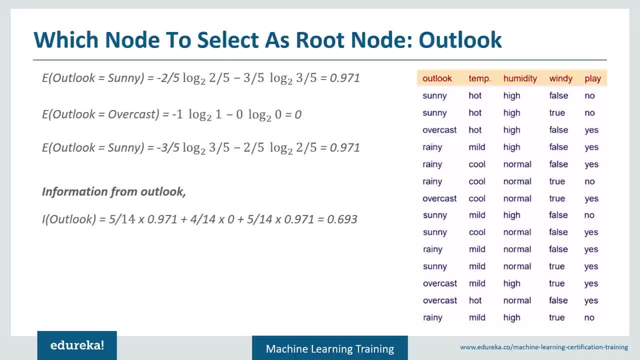 by entropy of each feature. All right, So, as calculated, the entropy for Sunny is 0.971, right, So what we'll do will multiply 5 by 14 with 0.971, right? Well, this was a calculation for information. 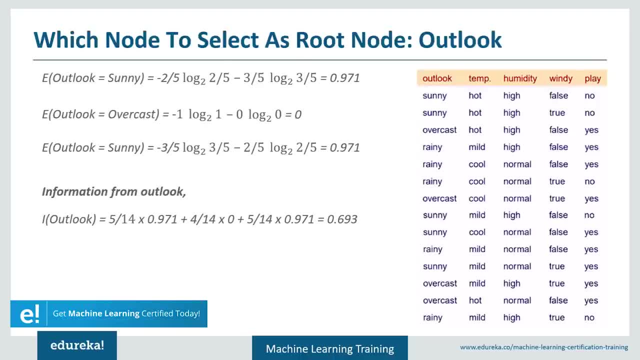 when Outlook equals Sunny, but Outlook even equals overcast and rainy, for in that case, What we'll do again similarly, will calculate for everything for overcast and Sunny. for overcast, weighted averages: 4 by 14, multiplied by its entropy, that is 0, and for Sunny it is same 5 by 14: 3.. 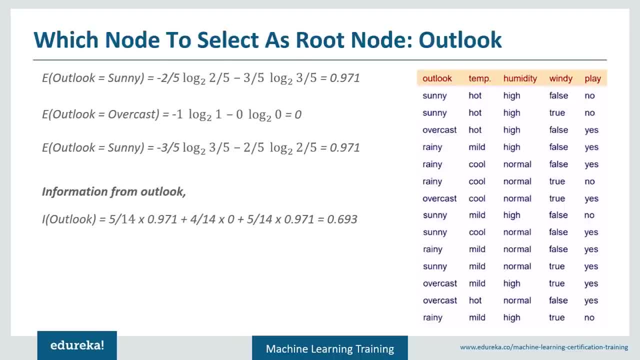 Yes and to knows, multiplied by its entropy, that is 0.971, and finally, will take the sum of all of them, which equals to 0.693. right next will calculate the information gained. this, what we did earlier was information taken from Outlook. Now we are calculating what is the information we are gaining. 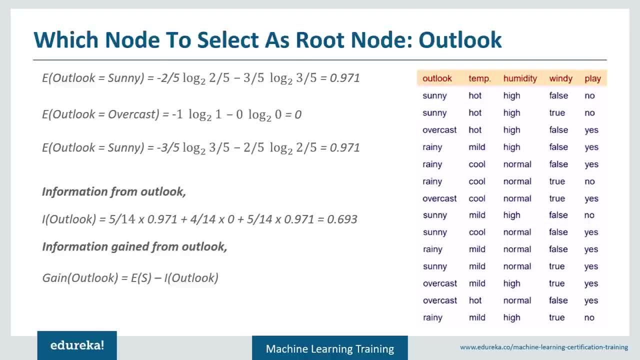 from Outlook. right now this information gain. that equals to total entropy minus the information that is taken from Outlook. All right, so total entropy- we had 0.94, minus information We took from Outlook- is 0.693.. So the value of information gained. 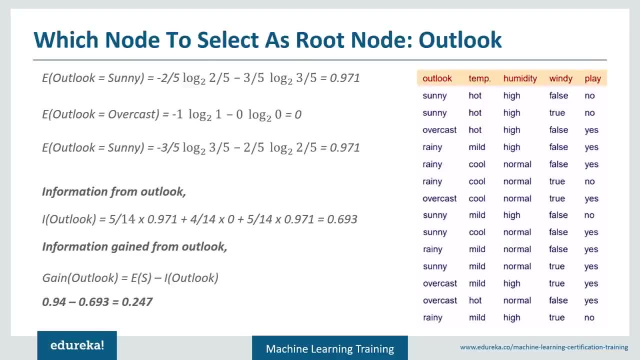 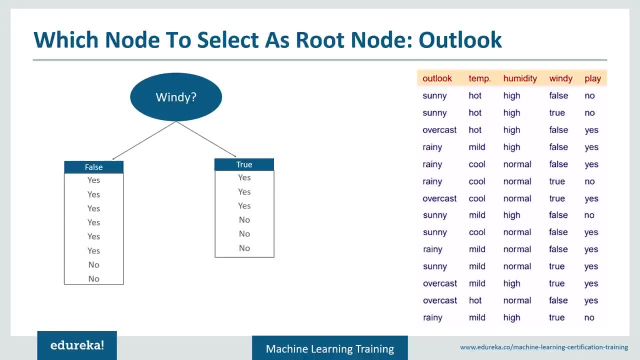 from Outlook results to 0.247.. All right, So next, what do we have to do? Let's assume that Wendy is our root node. So Wendy consists of two parameters: false and true. Let's see how many yes and how many knows are there? 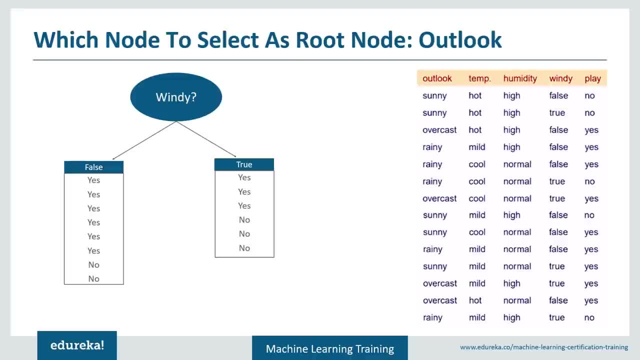 in case of true and false. So when Wendy has false as its parameter, then in that case it has six yes and two knows, and when it has true as its parameter, it has three years and three knows a light. So let's move ahead and similarly calculate the information taken from Wendy. 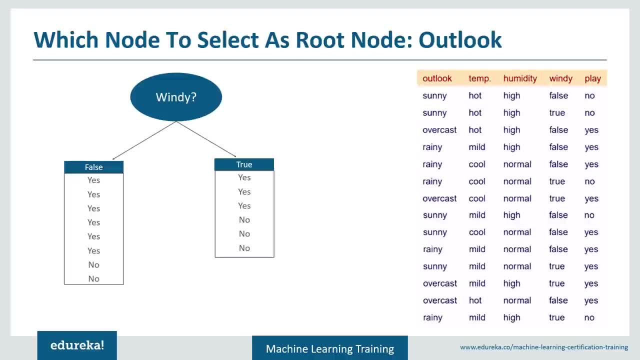 and finally calculate the information gained from Wendy. All right, So first of all, what we'll do will calculate the entropy of each feature, Starting with windy: equal, true. So in case of true, we had equal number of yes and equal number of no. will remember the graph. 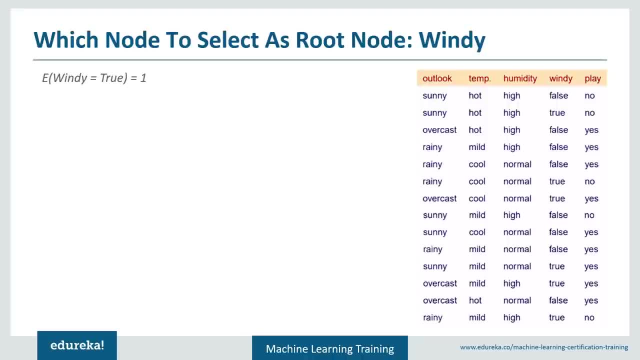 when we had the probability as 0.5, as total number of years equal total number of no, and for that case the entropy equals one. so we can directly write entropy of true when it's windy is one, as we had already proved it, when probability equals 0.5. 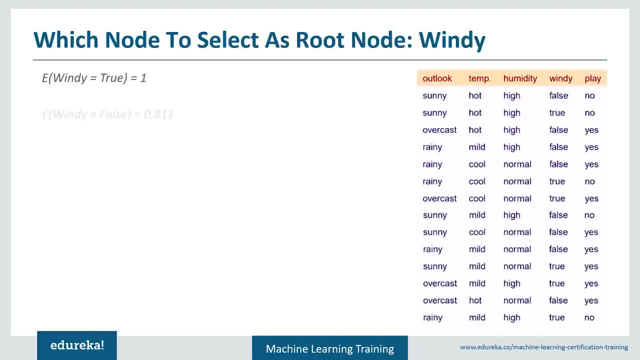 The entropy is the maximum that equals to one, All right. next is entropy of false when it is Wendy, All right. So, similarly, just put the probability of yes and no in the formula and then calculate the result, since you have six years and two knows. so in total, 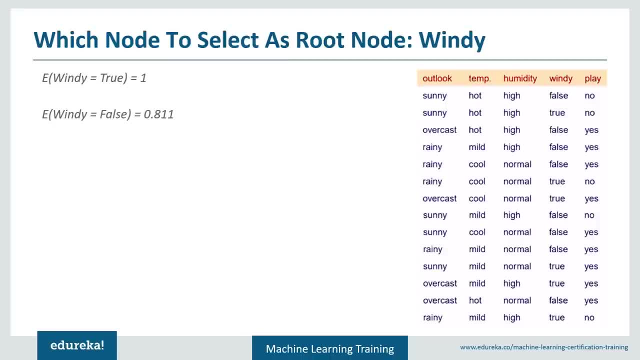 you'll get the probability of yes as 6 by 8 and probability of no as 2 by 8.. All right, So when you will calculate it, you will get the entropy of false as 0.811.. All right, Now let's calculate the information from Wendy. 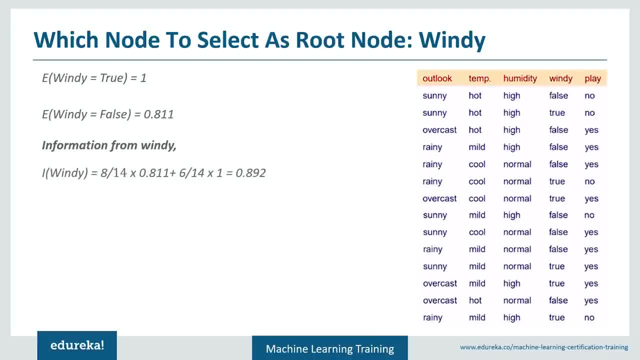 So total information collected from Wendy equals information taken when Wendy equal true, plus information Taken when Wendy equal false. So we'll calculate the weighted average for each one of them and then we'll sum it up to finally get the total information taken from Wendy. 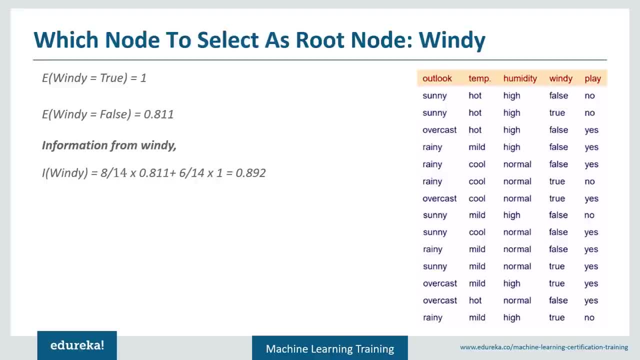 So in this case it equals to 8 by 14 multiplied by 0.811, plus 6 by 14 multiplied by 1.. What is this 8? it is total number of yes and no. in case when windy equals false right. 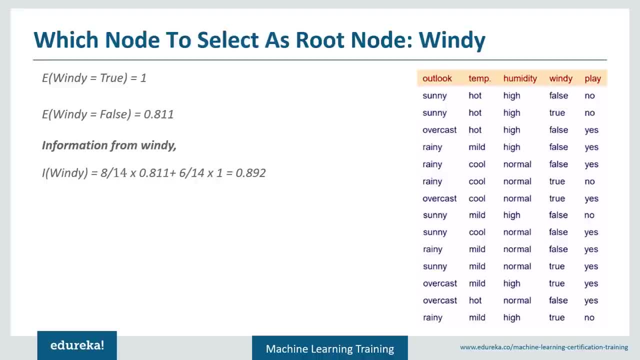 So when it was false. so total number of years: that equals to 6 and total number of no: that equal to 2, that sum ups to 8.. All right, So that is why the weighted Average results to 8 by 14. similarly, information taken. 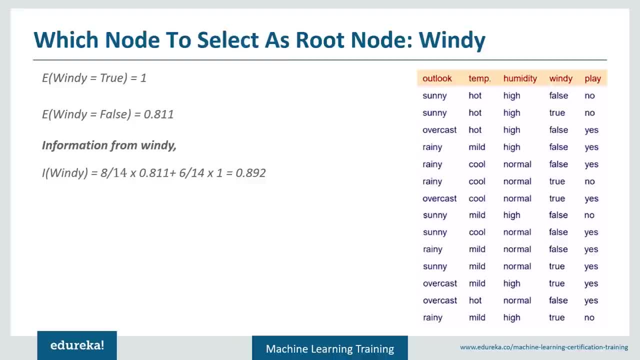 when windy equals true equals to 3 plus 3. that is, 3 yes and 3 no equals 6 divided by total number of sample space. That is 14 multiplied by 1. that is entropy of true. All right, so it is 8 by 14, multiplied by 0.811 plus 6. 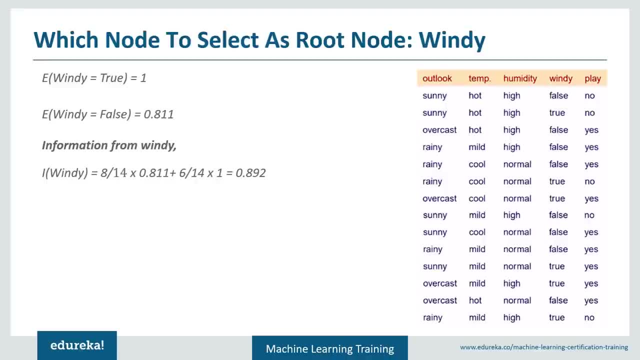 by 14, multiplied by 1, which results to 0.892.. This is information taken from Wendy. All right now, how much information you are gaining from Wendy. So for that, what you will do. so total information gained from Wendy that equals to total entropy minus information taken. 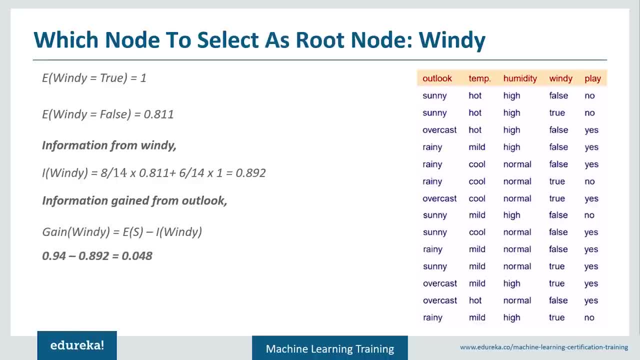 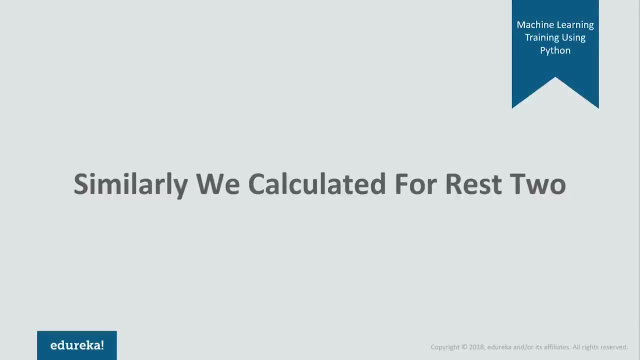 from Wendy All right. that is 0.94 minus 0.892. that equals to 0.048.. So 0.048 is the information gained from Wendy All right. Similarly, we calculated for the rest to all right. So for Outlook, as you can see, the information was 0.693. 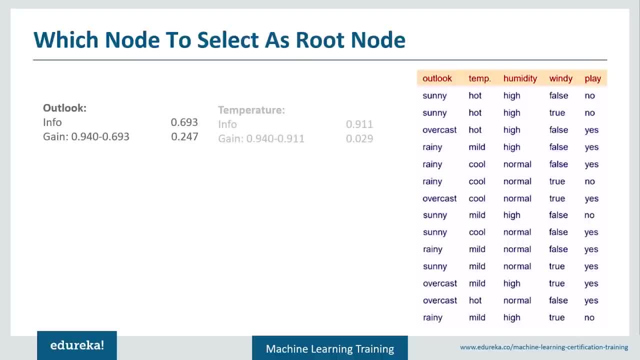 and its information gain was 0.247. in case of temperature, the information was around 0.911 and the information gain that was equal to 0.029. in case of humidity, the information gain was 0.152 and in the case of windy, the information gain was 0.048.. 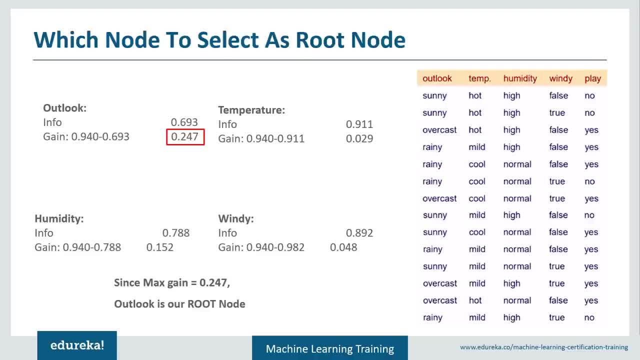 So what we'll do will select the attribute with the maximum mood. fine, Now we are selected Outlook as our root node, and it is further subdivided into three different parts: Sunny, overcast and rain. So in case of overcast, we have seen that it consists of all. 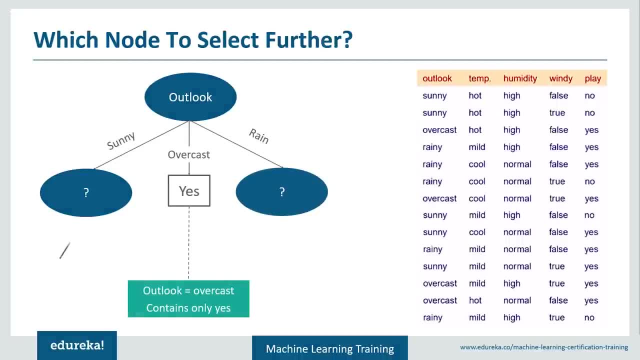 Yes, so we can consider it as a leaf node, But in case of Sunny and rainy it's doubtful, as it consists of both Yes and both know. so you need to recalculate the things right again for this node. You have to recalculate the things. 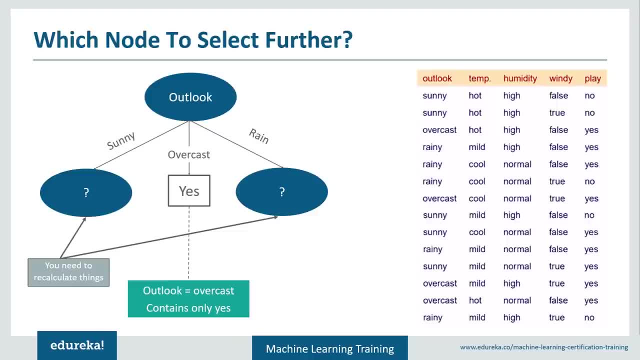 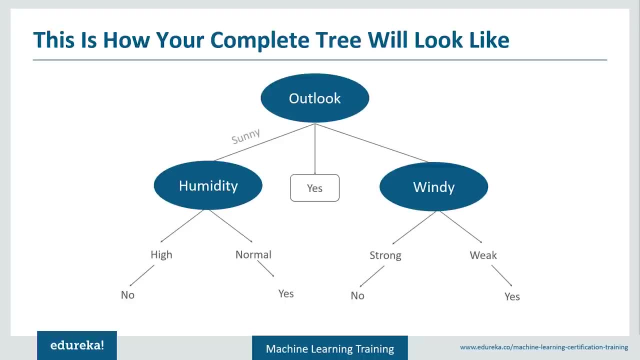 All right, you have to again select the attribute, which is having the maximum information gain. All right, So there's how your complete tree will look like a light. So let's see when you can play. So you can play when Outlook is overcast. 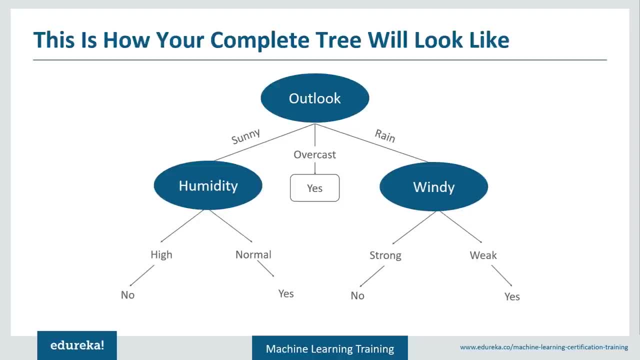 All right, in that case you can always play. if the Outlook is Sunny, you will further drill down to check the humidity condition. All right, if the humidity is normal, then you will play. if the humidity is high, then you won't play. right when the Outlook predicts. 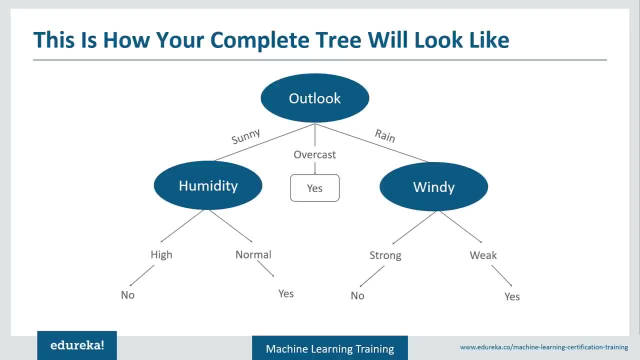 that it's rainy, then further you'll check whether it's windy or not. If it has a weak wind, then you'll go and opt for play, But if it has strong wind then you won't play right. So this is how your entire decision tree would look. 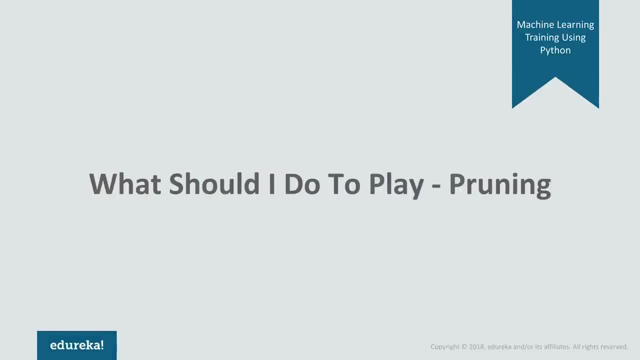 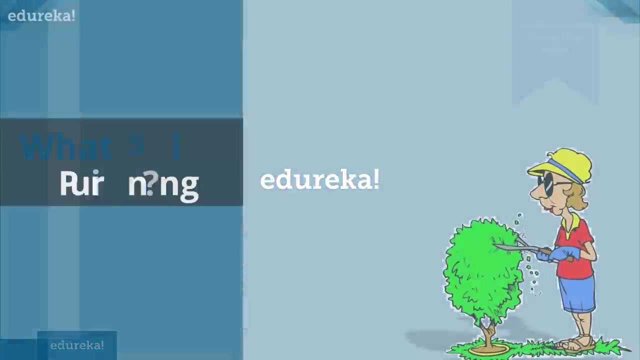 like at the end: All right, Okay, now comes the concept of pruning. says that: what should I do to play? Well, you have to do pruning. pruning will decide how you will play. What is this pruning? Well, this pruning is nothing but cutting down the nodes. 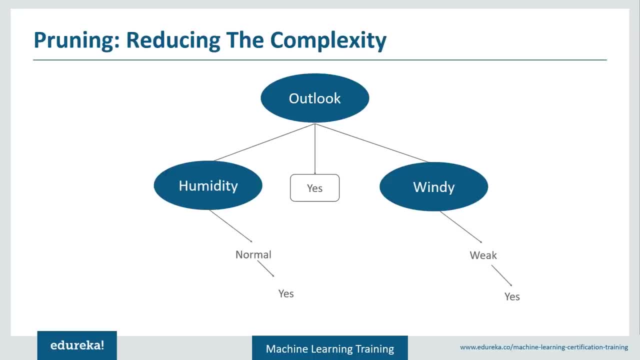 in order to get the optimal solution, All right. So what pruning does? it reduces the complexity, All right, as here. you can see on the screen that it's showing only the result for years. That is, it's showing all the results, Which says that you can play all right. 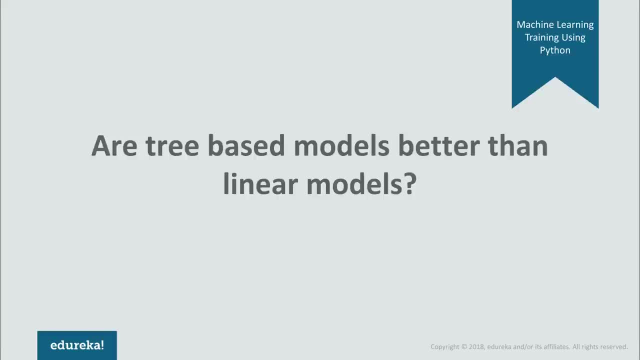 Before we drill down to a practical session, a common question might come in your mind. You might think that our tree based model better than linear model. right? You can think like: if I can use a logistic regression for classification problem and linear regression for regression problem, 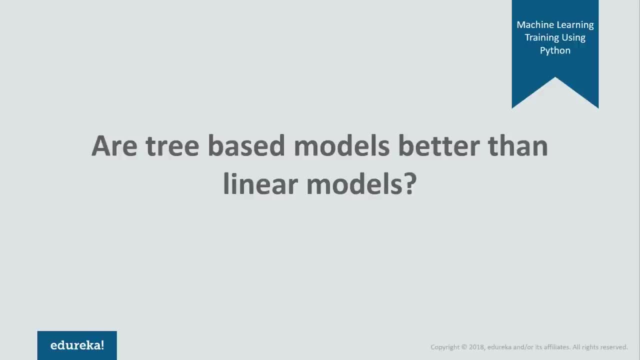 then why there is a need to use the tree. Well, many of us have this question in their mind, and well, there's a valid question. Question 2 will actually. as I said earlier, you can use any algorithm. It depends on the type of problem you're solving. 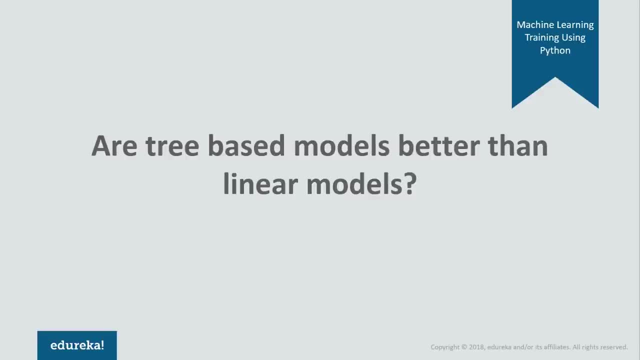 Let's look at some key factor which will help you to decide which algorithm to use and when. so the first point being: if the relationship between dependent and independent variable is well approximated by a linear model, then linear regression will outperform tree based model. second case: if there is a high non-linearity, 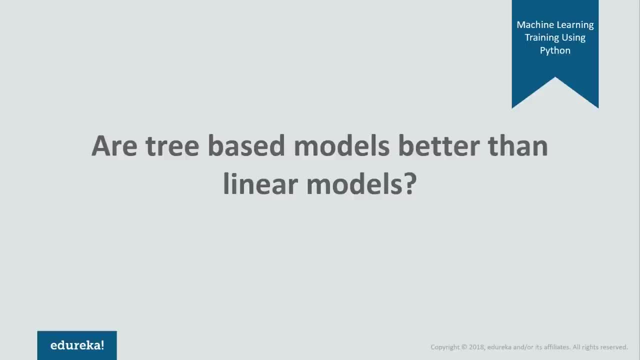 and complex relationship between dependent and independent variables, A tree model will outperform a classical regression model. and third case: if you need to build a model which is easy to explain to people, a decision tree model will always do better than a linear model, as the decision tree models are simpler to interpret. 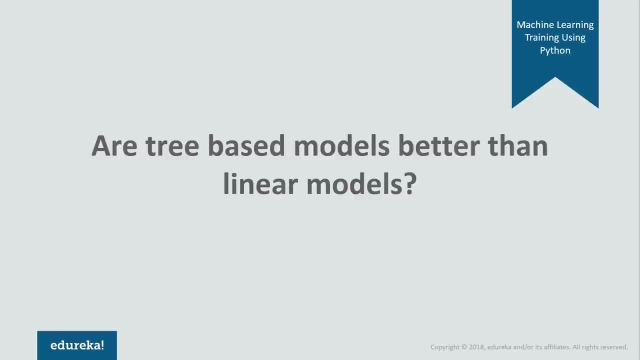 than linear regression. All right, Now let's move on ahead and see how you can write a decision tree classifier from scratch and python using the cart algorithm. All right, for this I'll be using Jupiter notebook with python 3.0 installed on it. 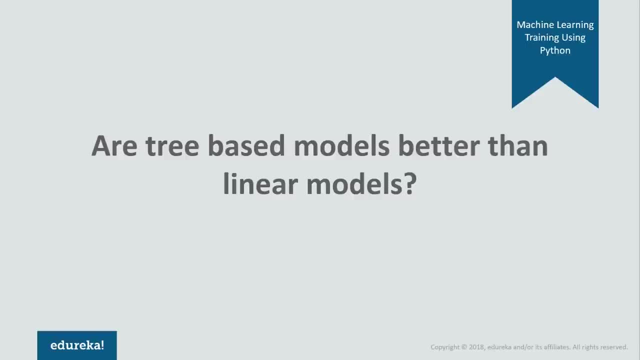 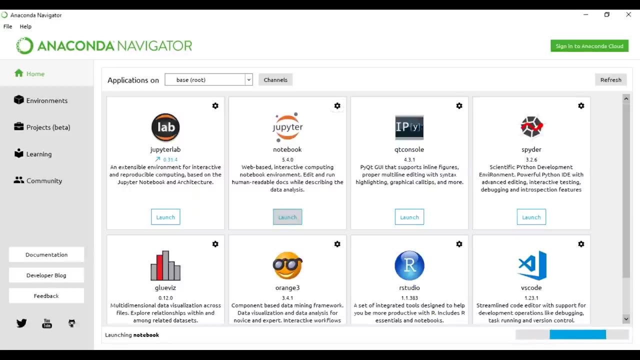 All right, So let's open the Anaconda and the Jupiter notebook. Where is that? So there's a anaconda Navigator and I'll directly jump over to Jupiter notebook and hit the launch button. I guess everyone knows that Jupiter notebook is a web-based. 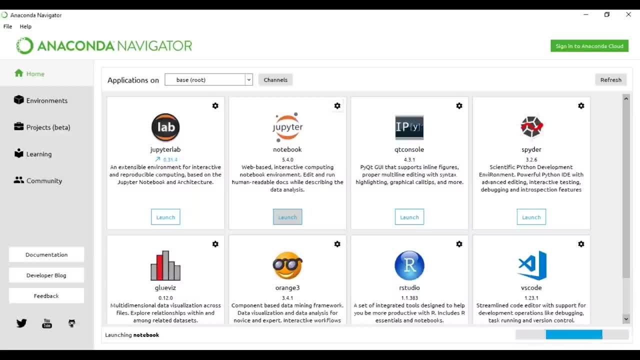 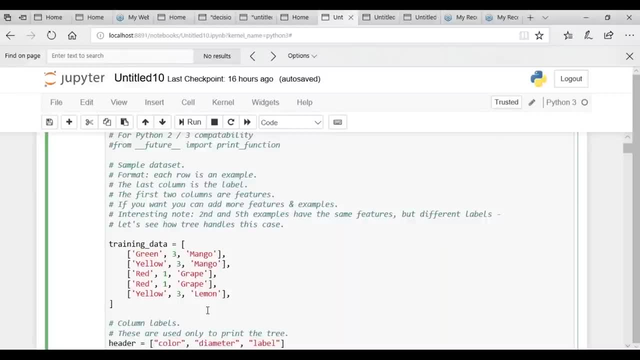 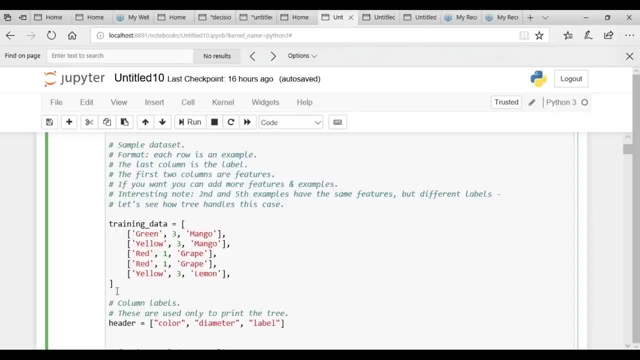 interactive computing notebook environment where you can run your python codes. So my Jupiter notebook. it opens on my localhost 8891.. So I'll be using this Jupiter notebook in order to write my decision tree classifier using python. for this decision tree classifier, I have already written the set of codes. 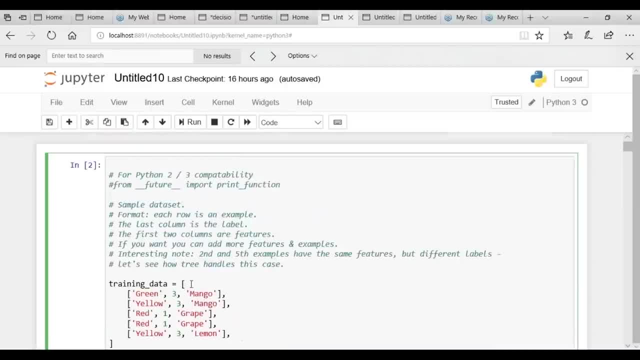 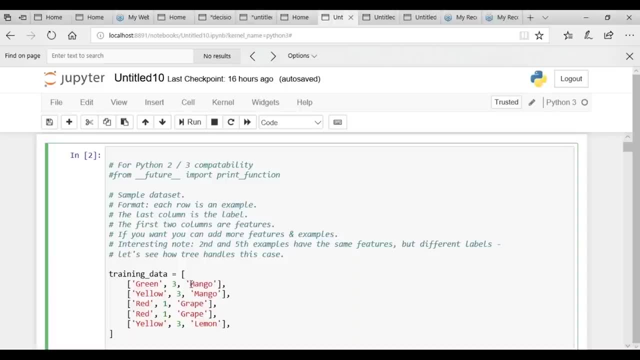 Let me explain you Just one by one. So we'll start with initializing our training data set. So there's a sample data set for which each row is an example. The last column is a label and the first two columns are the features. 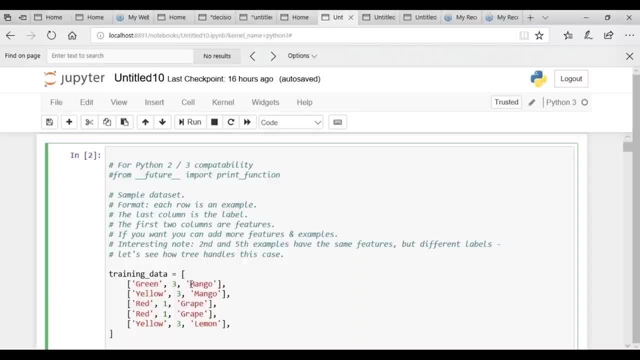 If you want, you can add some more features and example for your practice. Interesting fact is that this data set is designed in a way that the second and a fifth example have almost the same features, but they have different labels. All right, So let's move on and see how the tree handles this case. 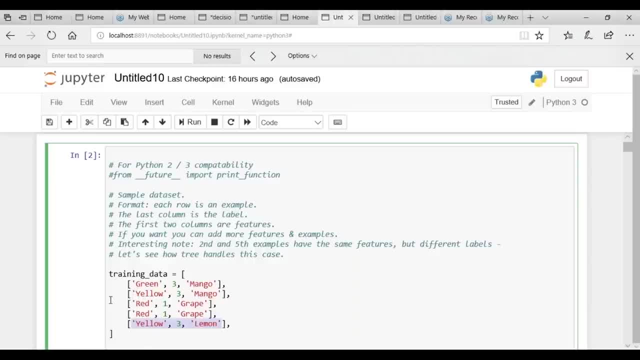 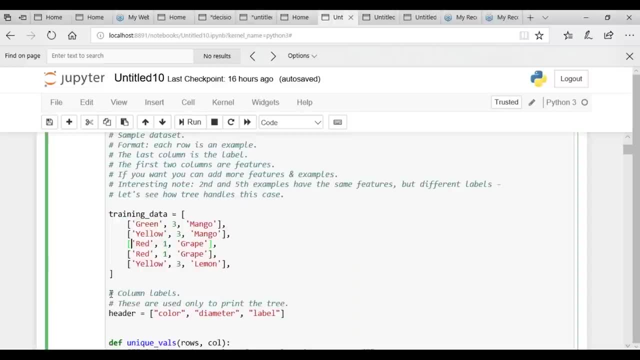 as you can see here, both of them- the second and the fifth column- have the same features. What the different is just their label. So let's move ahead. So this is our training data set. next, what we are doing, We are adding some column labels. 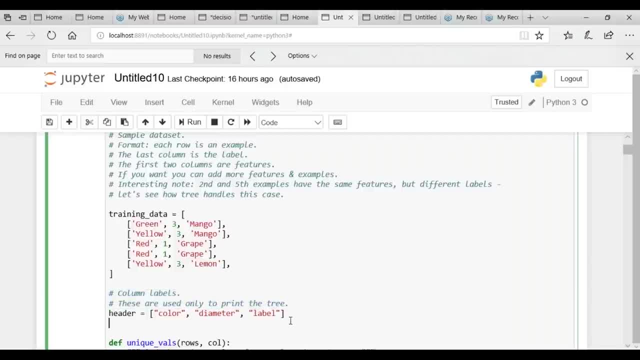 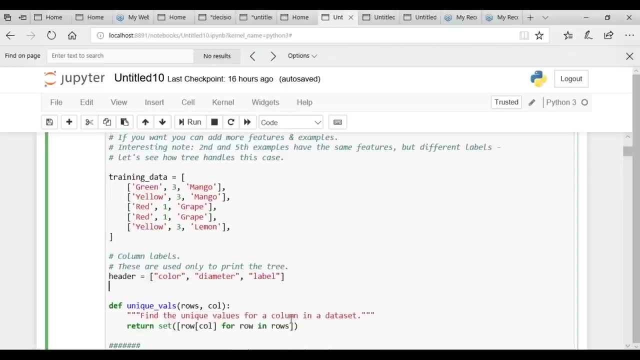 So they are used only to print the trees. fine, So what we'll do, we will add header to the columns, like the first column is of color, second is of diameter and third is of label column. All right, Next, what we'll do will define a function as unique values. 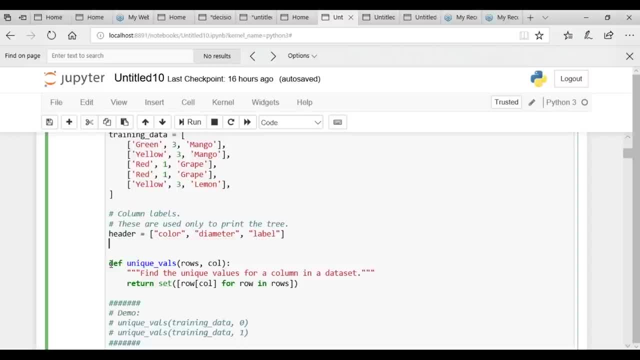 in which will pass the rows and the columns. So this function, what it will do: it will find the unique values for a column in the data set. So there's an example for that. So what we are doing here, we are passing training data as our own and column number as 0.. 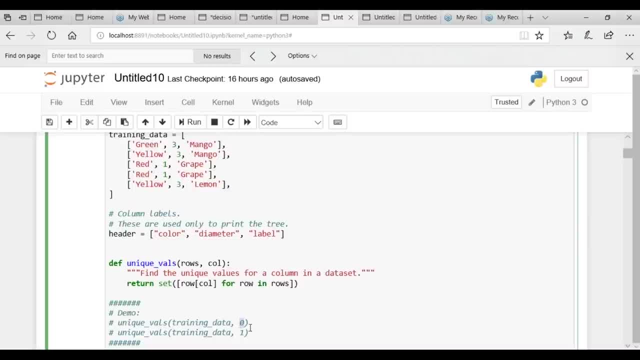 So what we are doing, we are finding unique values in terms of color and in this, since the row is training data and the column is one, So what you are doing here? so we are finding the unique values in terms of diameter, fine. So this is just an example. next, what we'll do, will define. 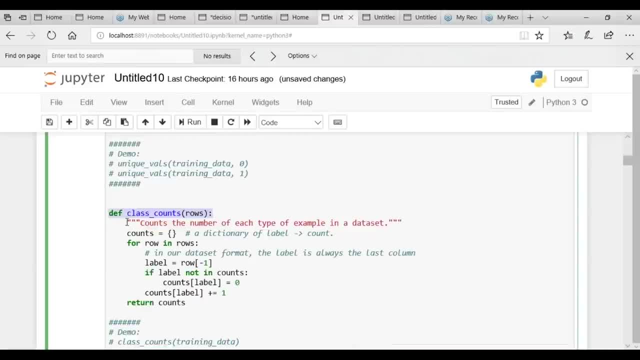 a function as class count and will pass the rows into it. So what it does, it counts the number of each type of example within data set. So in this function, what we are basically doing, we are counting the number of each type, for example, in the data set. or what we are doing. 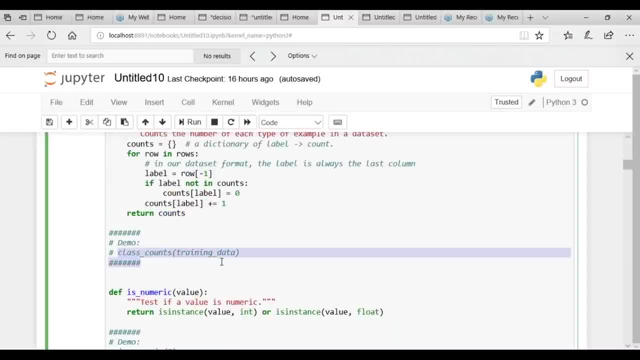 We are counting the unique values for the label in the data set. as a sample You can see here. we can pass that entire training data set to this particular function as class underscore count. what it will do: it will find all the different types of label within the training data set. as you can see here the unique. 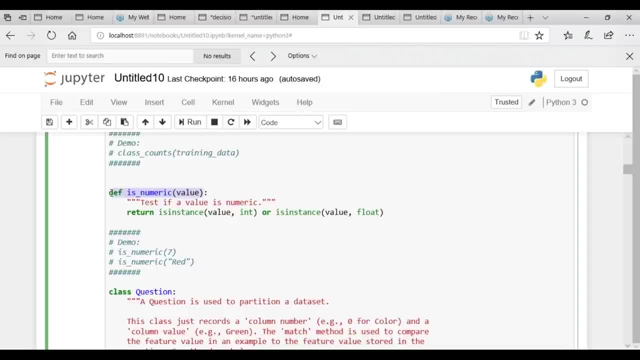 label consists of mango grape and lemon. So next, what we'll do will define a function is numeric and will pass our value into it. So what it will do, It will just test if the value is numeric or not and it will return if the value is an integer or a float. 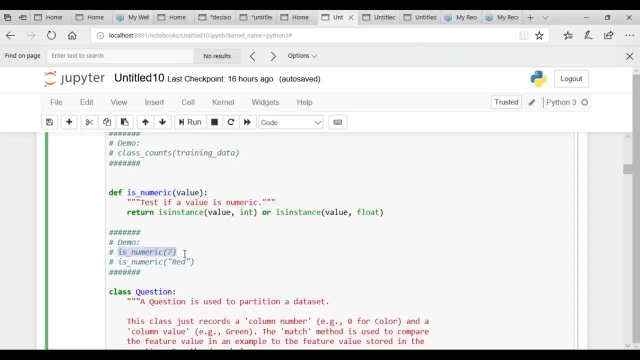 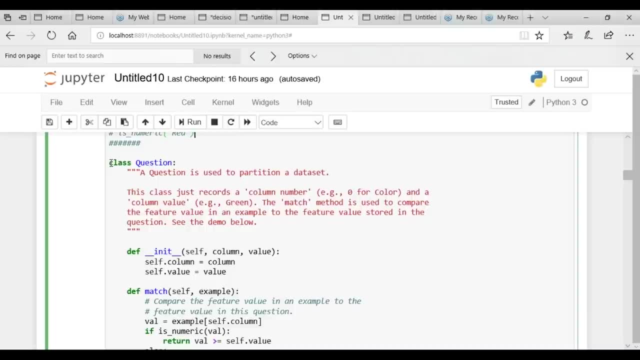 For example you can see, is numeric. we are passing seven, So it has an integer, So it will return an int value, and if you are passing red, it's not a numeric value, right? So moving on ahead will define a class named as question. 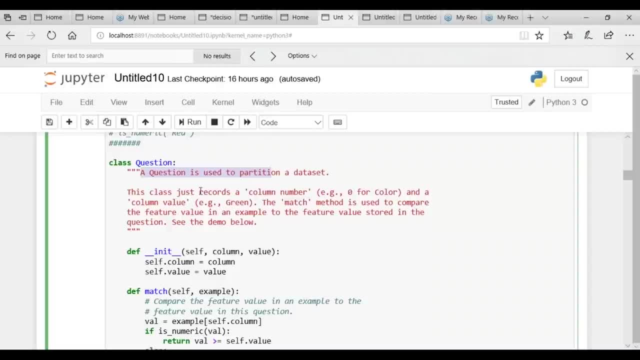 So what this question does? this question is used to partition the data set, this class. what it does? It just records a column number, for example 0, for color or light, and a column value, for example green. next, What we are doing, We are defining a match method which is used to compare. 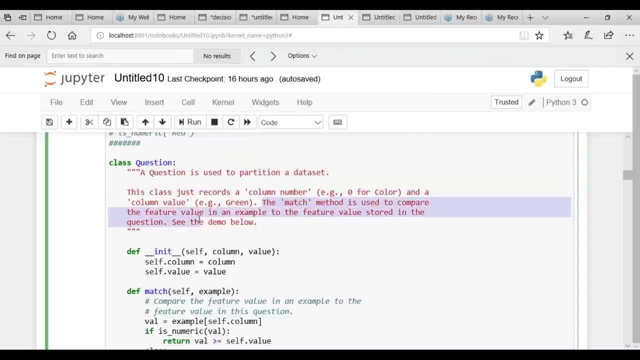 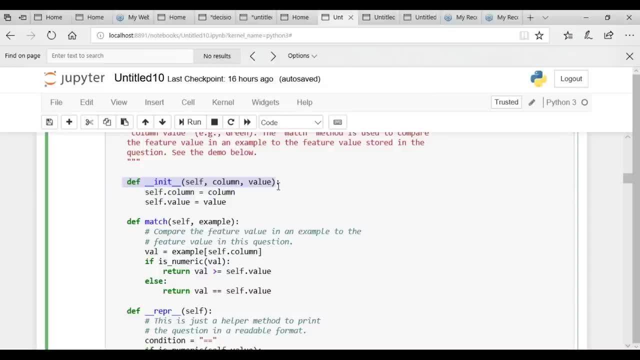 the feature value in the example to the feature value stored in the question. Let's see how. first of all, what we are doing. We're defining an init function and inside that we are passing the self column and the value as parameter. So next, what we do. we define a function as match what it does. 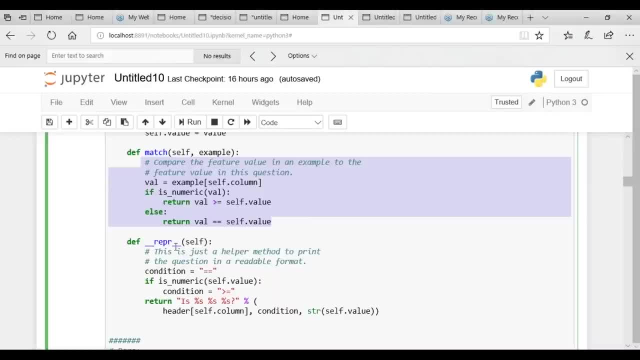 it compares the feature value in an example to the feature value in this question. When next we'll define a function as our EPR, which is just a helper method to print the question in a readable format, Next, what we are doing: We are defining a function, partition. 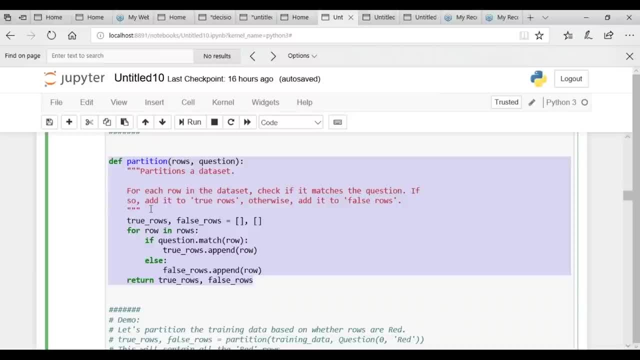 Well, this function is used to partition the data set. each row in the data set It checks if it matches the question or not. if it does so, it adds it to the true rows, or if not, then it adds to the false rows. All right, for example, 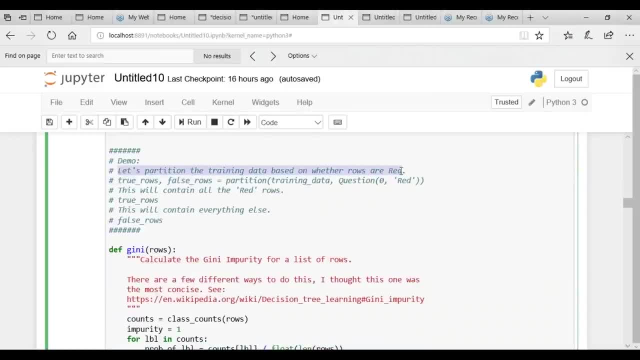 as you can see here, let's partition the training data set based on whether the rows are red or not. here We are calling the function question and we are passing a value of 0 and red to it. So what it will do? it will assign all the red Rose to true. 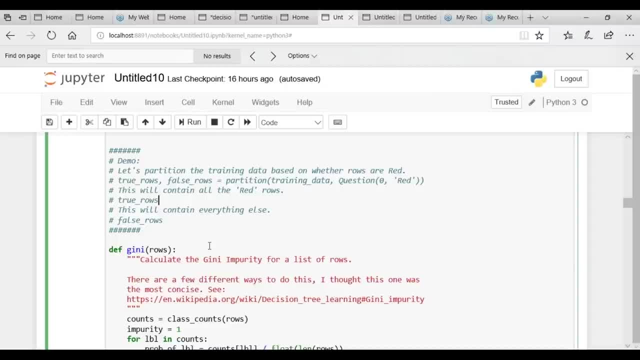 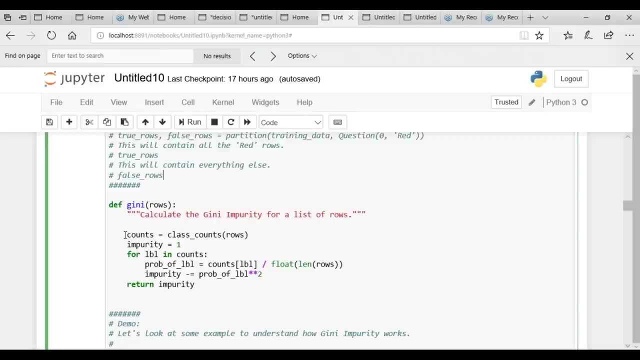 underscore Rose and everything else will be assigned to false underscore Rose. fine, Next, what we'll do will define a genie impurity function and inside that will pass the list of Rose. So what it will do, it will just calculate the genie impurity for the list of Rose. 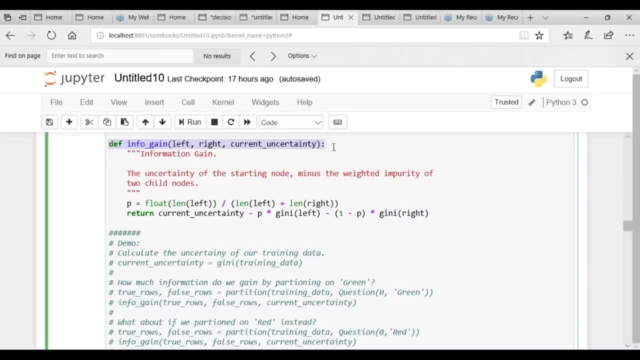 Next what we are doing here with defining a function as information gain. So what this information gain function does? it calculates the information gain using the uncertainty of the starting node minus the weighted impurity of the child node. The next function is find the best split. 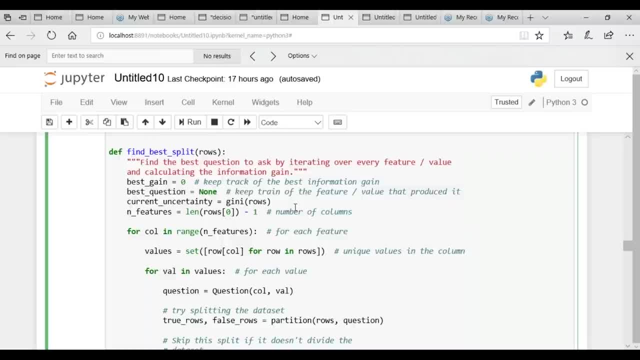 Well, this function is used to find the best question to ask by iterating over every feature or value and then calculating the information gain. for the detail explanation on the code, You can find the code in the description given below. All right, Next we'll define a class as leaf for classifying the data. 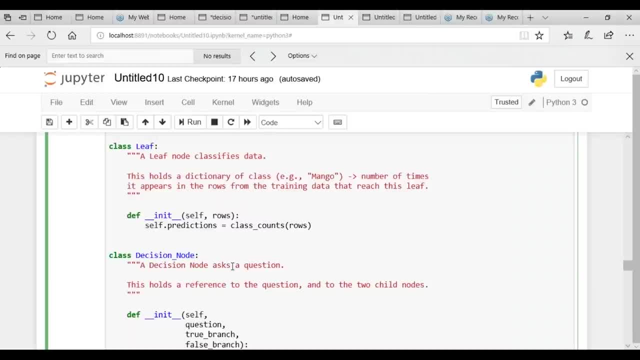 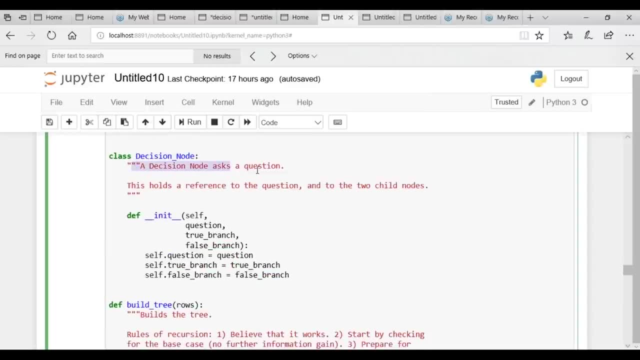 It holds a dictionary of class, like mango, for how many times it appears in the row from the training data that reaches the sleeve? All right, Next is the decision node. So this decision node, it will ask a question. This holds a reference to the question and the two child. 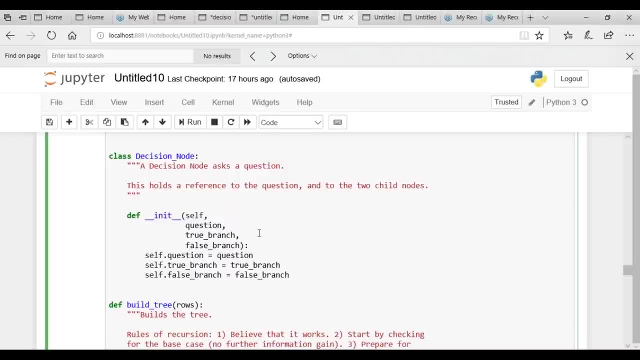 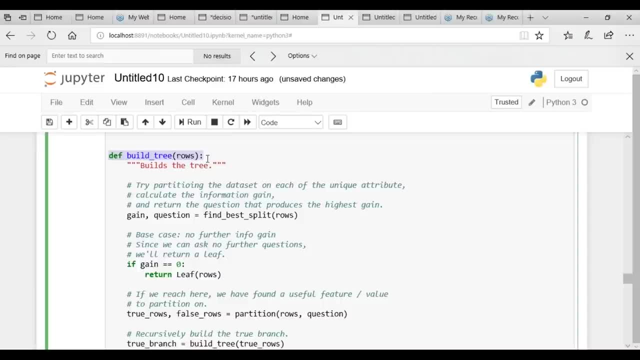 nodes. on the base of it, You are deciding which node to add further to which branch. All right, So next, what we are doing? we are defining a function of build tree and inside that we are passing our number of rows. So this is the function that is used to build a tree. 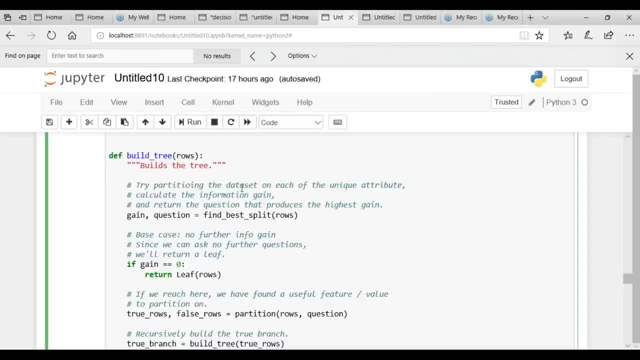 So, initially, what we did. we define all the various function that we will be using in order to build a tree. So let's start by partitioning the data set for each unique attribute. then we'll calculate the information gain And then return the question that produces the highest gain. 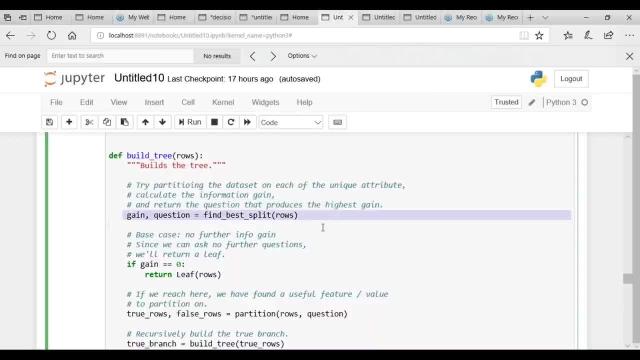 and, on the basis of that, will split the tree. So what we are doing here, We are partitioning the data set, calculating the information gain and then what this is returning. It is returning the question that is producing the highest gain. All right, 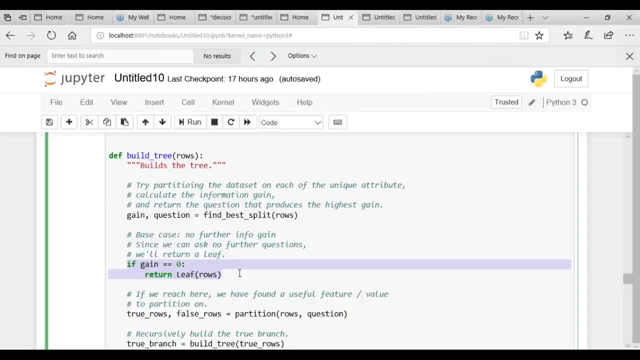 Now, if gain equals zero, return leaf rows. so what it will do? So if we are getting no for the gain, that is, gain equals zero, then in that case, since no further question could be asked, So what it will do? it will return a leaf, fine. 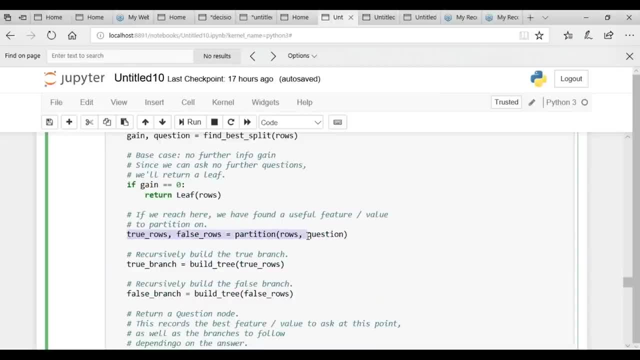 Now true underscore rows of false underscore rows, equal partition with rows, and the question: So if we are reaching till this position, then you have already found a feature of value which will be used to partition the data set. then what you will do? you will recursively build the. 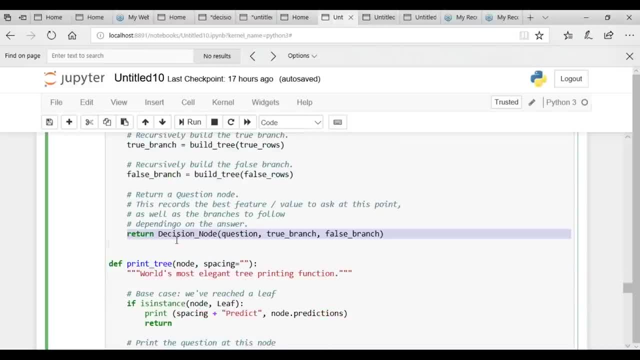 true branch and similarly recursively build the false branch. So return decision underscore node and inside that will be passing question: true branch and false branch. So what it will do, it will return a question node and this question node. this records the best feature or the value to 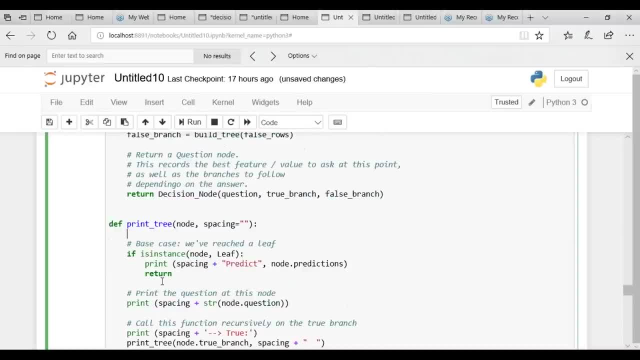 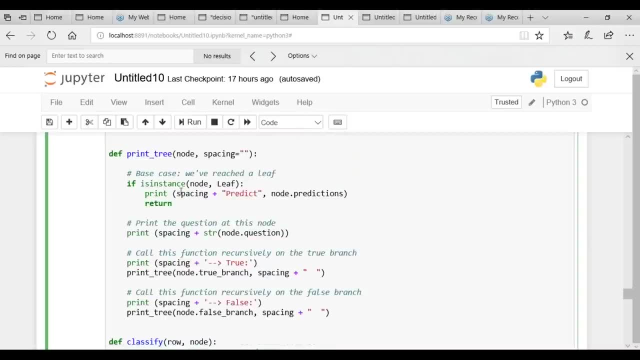 ask at this point: fine, Now that we have build our tree. next, what we'll do will define a print underscore tree function which will be used to print the tree. fine, So, finally, what we are doing in this particular function that we are printing our tree next is the classify function, which 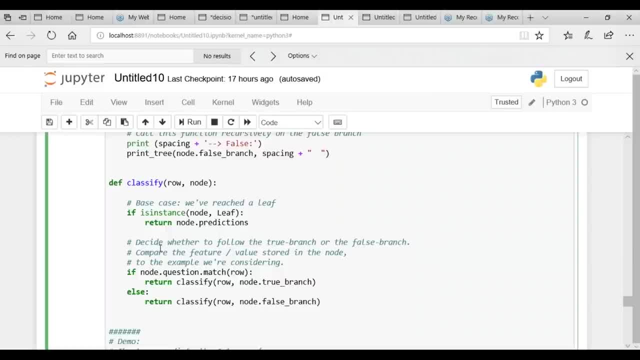 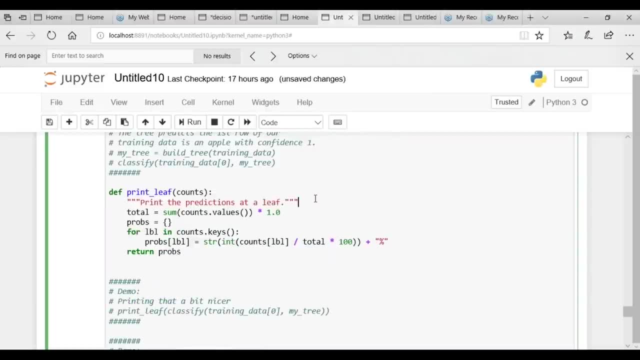 will use it to decide whether to follow the true branch or the false branch, and then compare to the feature of values stored in the node, to the example We are considering. and last, what we'll do will finally print the production and leave. So let's execute it. 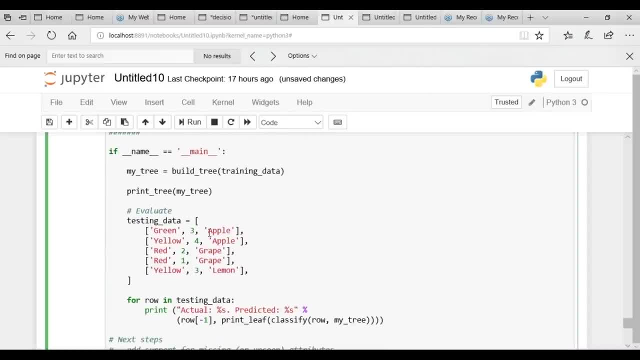 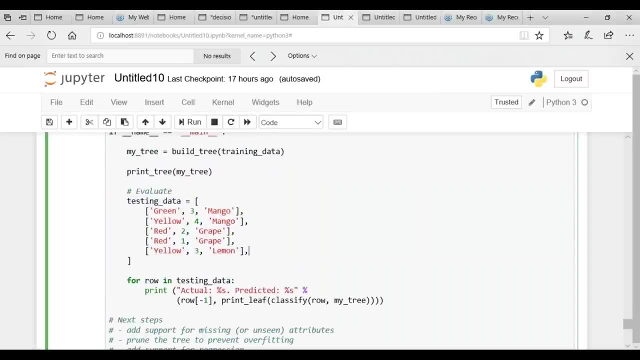 And see: okay, so there's our testing data. All right, so we printed our leaf as well. Now that we have trained our algorithm with our training data set, now it's time to test it. So there's our testing data set. 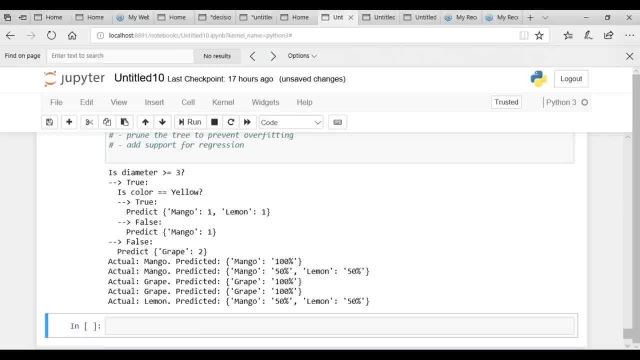 So let's finally execute it and see what is the result. So this is the result you will get. so first question which is asked by the algorithm is: is diameter greater than equal to 3? if it is true, then it will further ask if the color is. 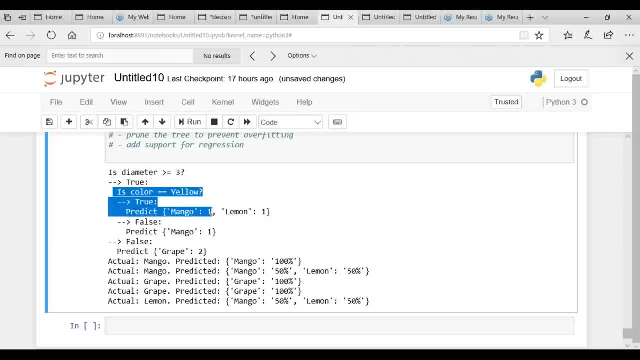 yellow Again. if it is true, then it will predict mango as one and lemon with one, All right, and in case it is false, then it will just predict the mango. Now, this was the true part. Now, next coming to, diameter is not greater than or equal to: 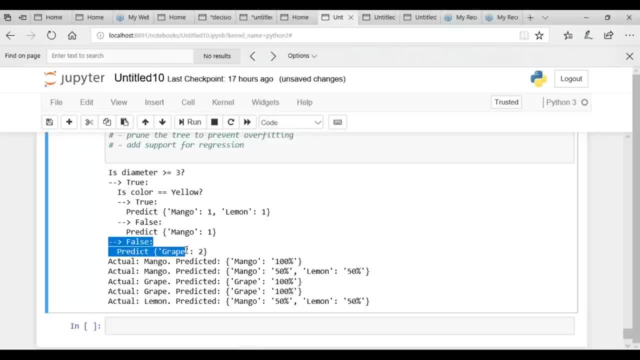 3, then in that case it's false. and what it will do? It will just predict the grape. fine, Okay, So this was all about the coding part. Now let's conclude this session. But before concluding, let me just show you one more thing. 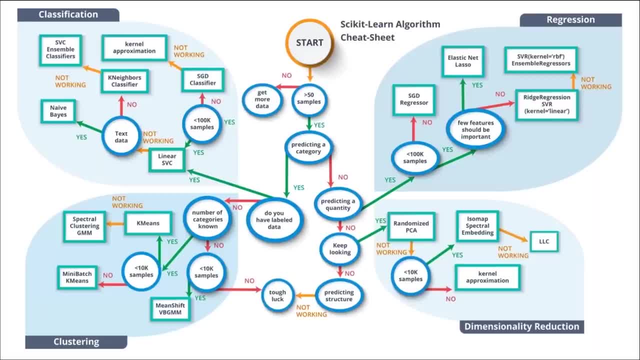 Now There's a scikit-learn Algorithm cheat sheet which explains you which algorithm you should use and when. all it it's built in a decision tree format. Let's see how it is built. So, first condition: it will check whether you have 50 samples. 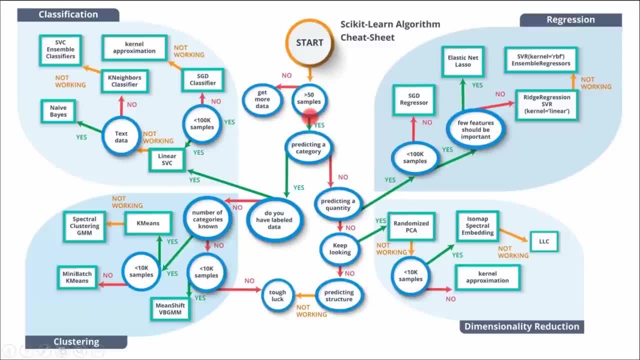 or not. If your samples are greater than 50, then it will move ahead. If it is less than 50, then you need to collect more data. If your sample is greater than 50, then you have to decide whether you want to predict a category or not. 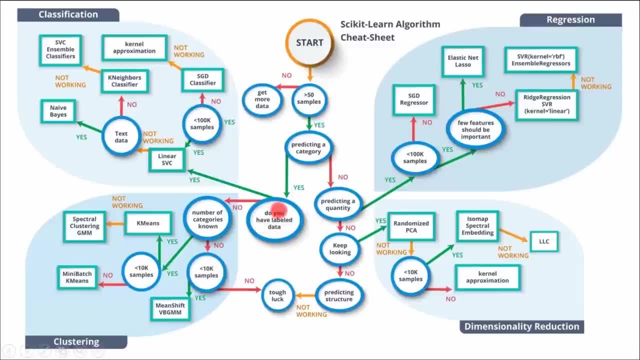 If you want to predict a category, then further you will see that whether you have labeled data or not. If you have labeled data, then that would be a classical classification algorithm problem. If you don't have the label data, then it would be a.